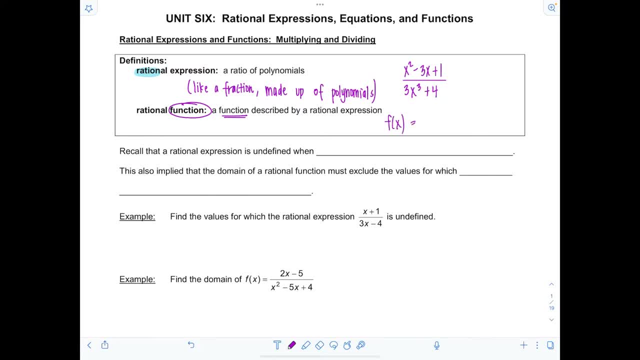 as f of x, right, since it's a function using our function notation. and then I would have that function equal to some sort of rational expression. okay, So expression right here. all by itself, function has f of x, equals the rational expression. All right, so far, so good. 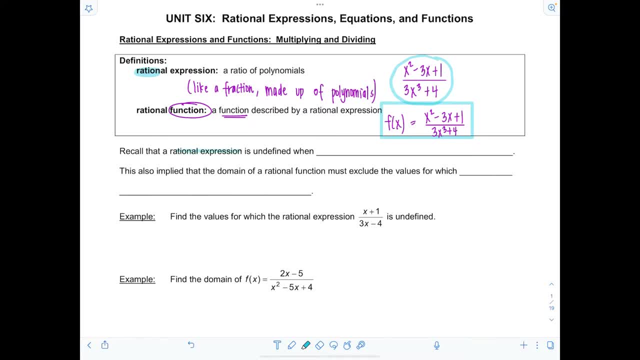 Lovely. Now, a rational expression is undefined when the denominator is 0. And remember, we are not allowed to divide by 0. So if the denominator of a rational expression is 0, it's undefined. This also implied that the domain of a rational function must exclude the values for which 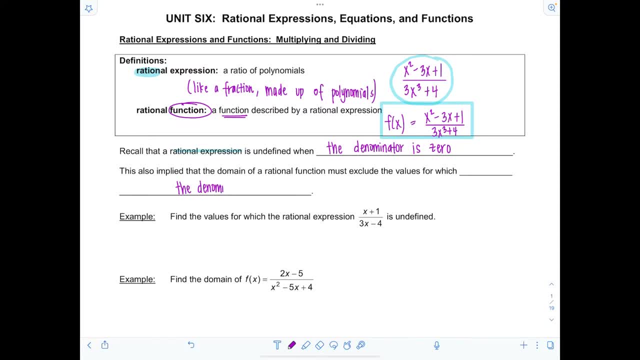 the denominator is 0. So essentially, you're always going to be interested in figuring out when the denominator is 0. If you're only talking about a rational expression, then you find where it's undefined. If you're talking about a rational function, then you 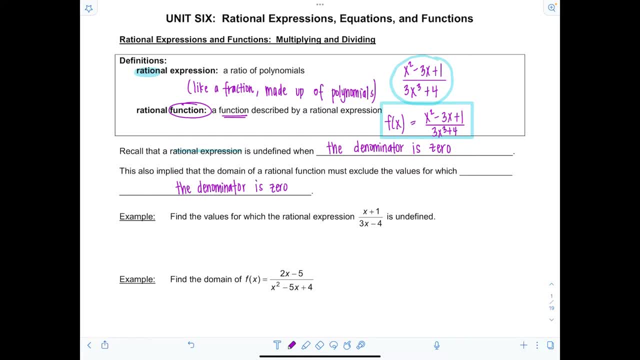 list the domain by specifying what the restrictions are. I'll show you exactly what I'm talking about. So first example says: find the values for which the rational expression x plus 1 over 3x minus 4 is undefined, Undefined. So remember: 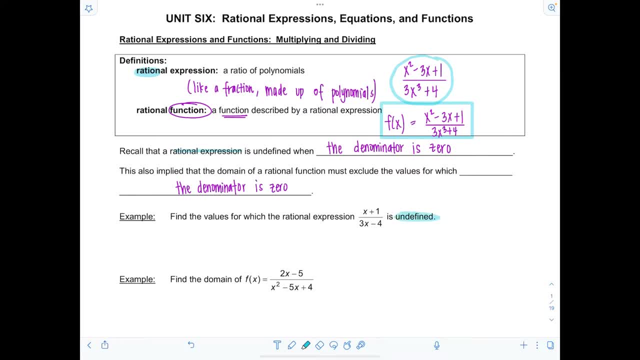 we are interested in particularly what values would make the denominator 0,, since that's where a rational expression would be undefined. I'm not interested in looking at the numerator When I'm finding where a rational expression is undefined. I just got to focus on. 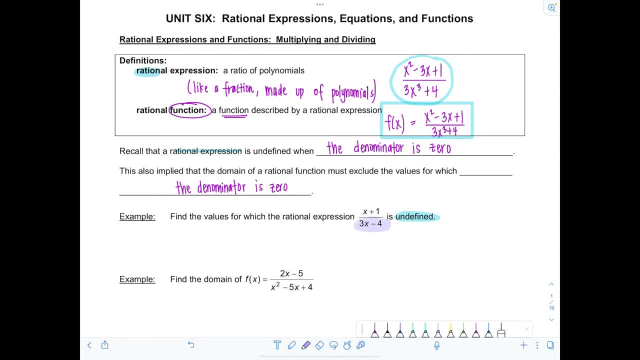 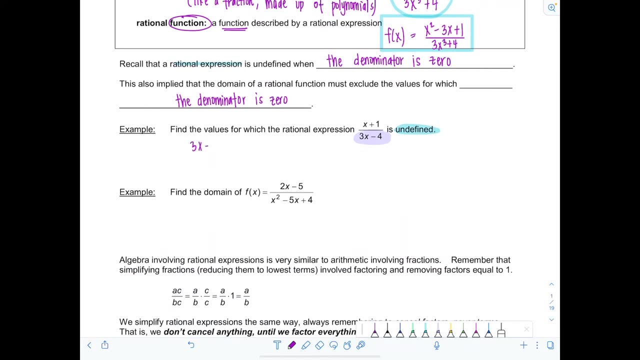 what is going on downstairs right here. So to figure out what would make 3x minus 4 equals 0, you can maybe just look at it and tell. Some of you are pretty quick like that. If you can't tell just by looking, then you're going to set it equal to 0, right? This is what we don't want. 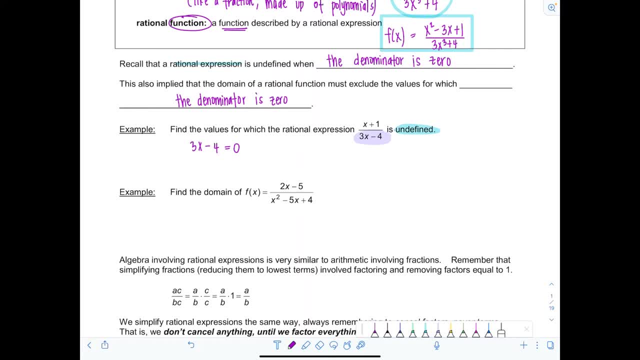 to happen and then solve for x. So we would add 4 to both sides. That gives us 3x is equal to 4.. So if x is 4 thirds, then the denominator is 0. So that tells me this rational expression is: 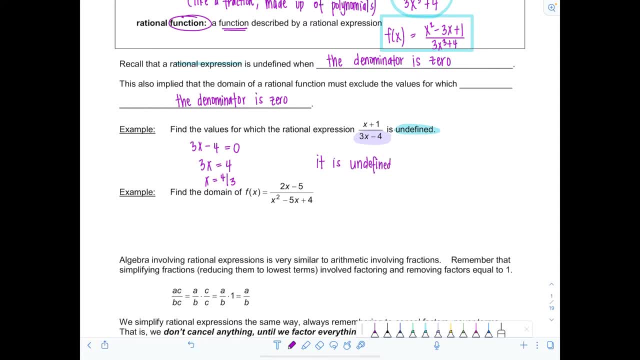 undefined At x equals 4 thirds. All right, Now, phrasing the question a little differently, we're asked to find the domain of a function, a rational function. in this case, f of x equals 2x minus 5 over x squared minus 5x. 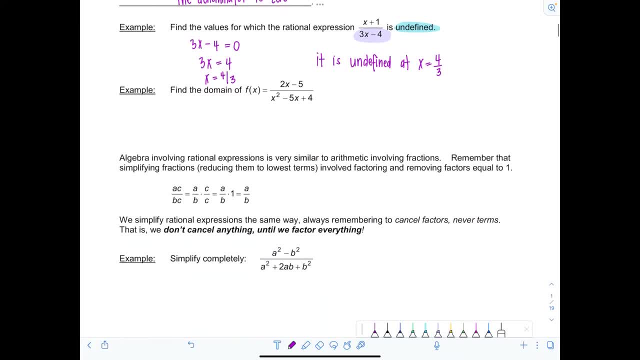 plus 4.. So again, just focus straight On the denominator when you're finding the domain for a rational function. And what I don't want is for x squared minus 5x plus 4 to equal 0. So let's see what the problem 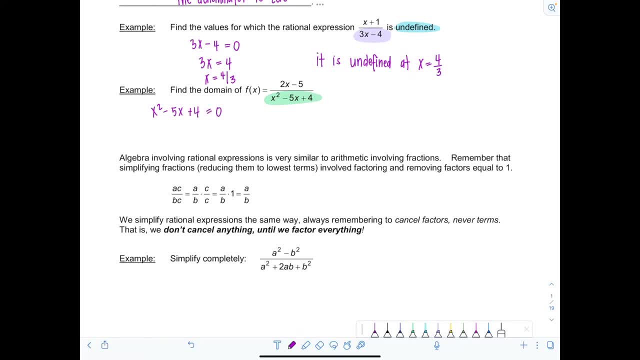 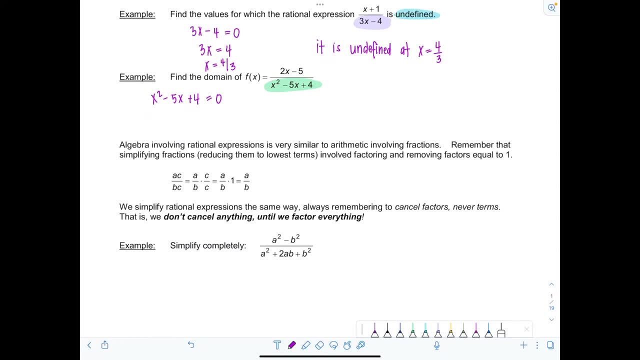 child values of x would be right. This is what we don't want to happen. Can I solve for x and see what values of x are going to be problematic for us? Well, we can factor this equation. It's going to factor into x minus 4 times x minus 4.. And it'll be equal to 0.. So what's going to happen is: 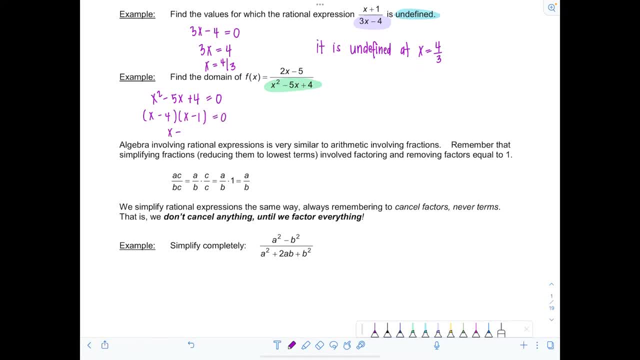 we're going to solve for x and see what values of x are going to be problematic for us. Well, we can factor this equation. It's going to factor into x minus 4, times x minus 4, times x minus 4.. one equals zero and our solutions are: x equals one and four. But remember, these x values are: 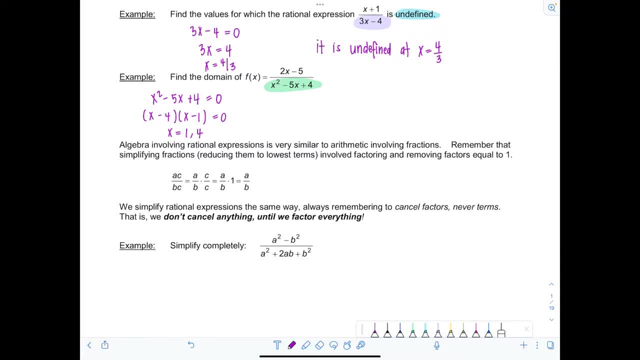 actually restrictions to our domain. This is what we do not want x to equal, because it would make the function undefined. So now, when we list our domain, easiest way to do it is using set builder notation, and you would say: our domain is the set of all x values, such that x does not equal. 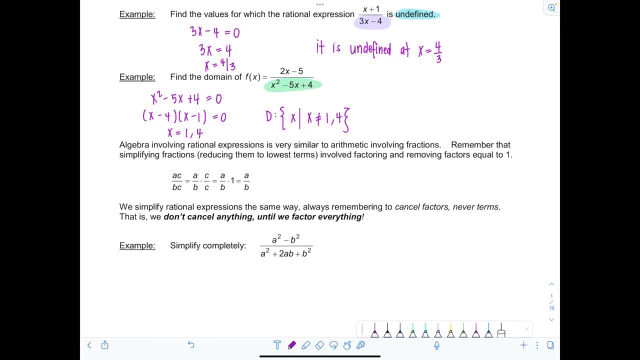 one or four, And when you write out your domain in this way, it's implied that all other values that x could take on in the real number system are good to go. You just have to list the ones that are no-no's, the restrictions, the ones that would make it undefined. Good, Now we're going to. 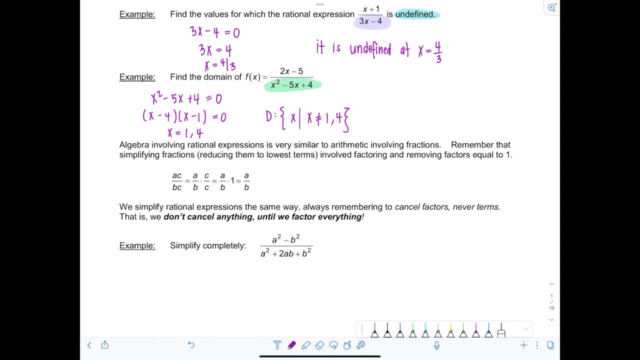 look at how to set builder So you simplify, multiply and divide rational expressions and functions, And it's always helpful to go back to our basic rules for arithmetic and dealing with rational numbers to come up with our rules for how to work with rational expressions. 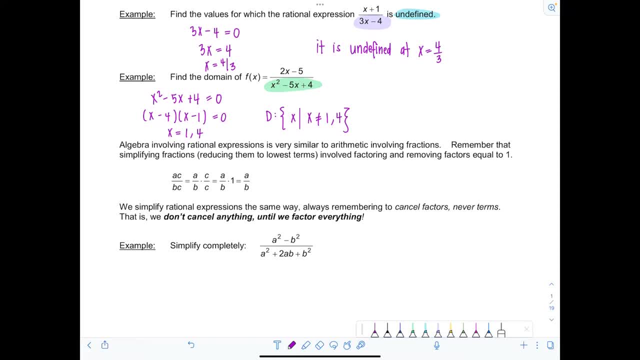 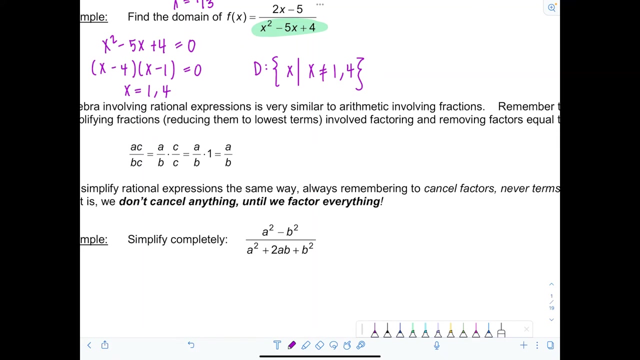 So remember that when you're simplifying a fraction, when you're reducing it to lowest terms, the best way to do it is you factor the numerator, factor the denominator and you cancel out or remove factors that are equal to one. So here's just a general example: If you have a times c over b times c, you can rewrite that. 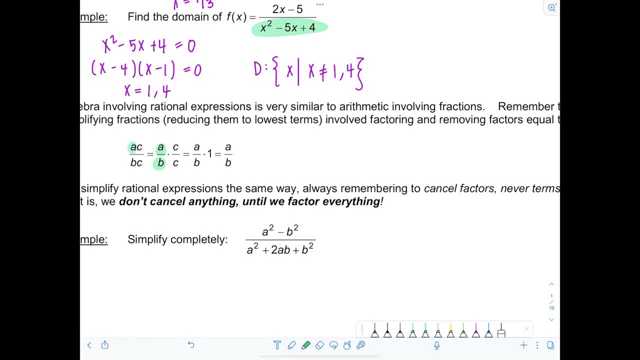 rational expression as a divided by b, grouping these two terms together, times, and then you separate out c over c here, which is just one, which is why it cancels, or you can remove it from the expression. So, for example, let me give you something we can kind of play around with. 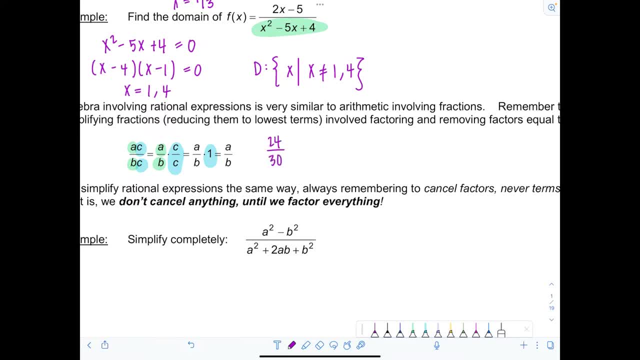 Say you had 24 over 30, right? So the best way to simplify or reduce this is remove any common factors that they have. So I noticed 6 goes into both 24 and 30. So I could write this as 4 times 6 over 5 times 6.. 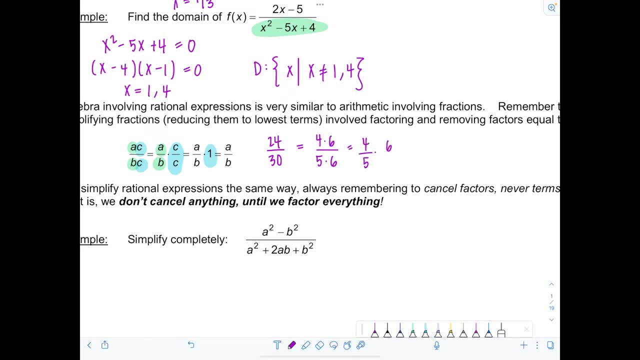 Remove the factor of 6 from the top and bottom And write it as 6 over 6.. over six, which is four over five times, this guy is now a one, which is why we're just left with four-fifths. I mean, usually we don't sit there and write all. 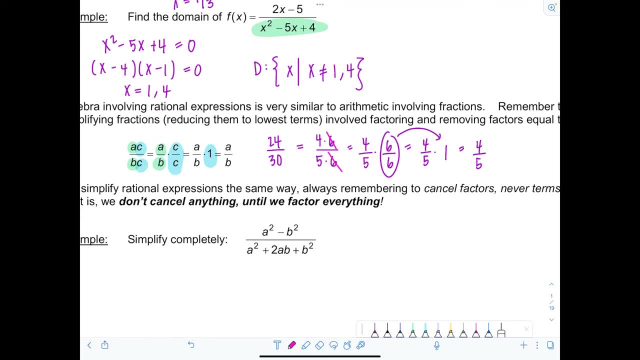 that out right. usually, you just go bam bam, cancel out the sixes and you go straight to four-fifths, but that's basically what's going on behind the scenes, so same thing is gonna happen with our rational expressions. the important thing, though, is that you have to wait until everything is factored. 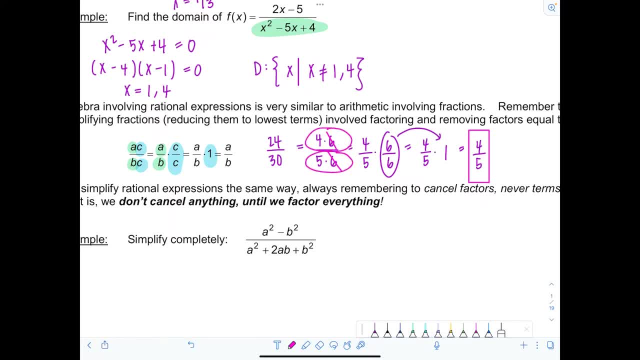 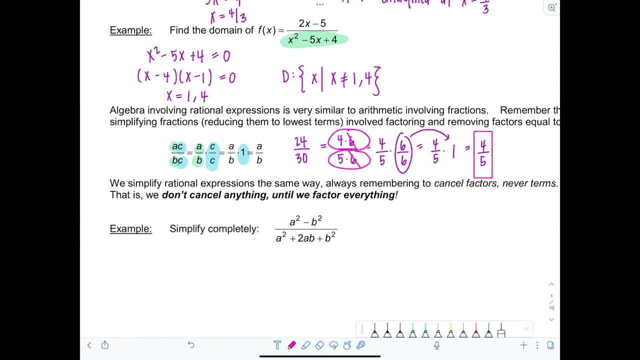 before you can cancel. okay, so when you have 24 over 30, you can't start canceling until you've factored the numerator, factor, the denominator. maybe you do it mentally with rational expressions. we're gonna actually write out all the factoring, okay, so I got this in bold for you here: we do not cancel. 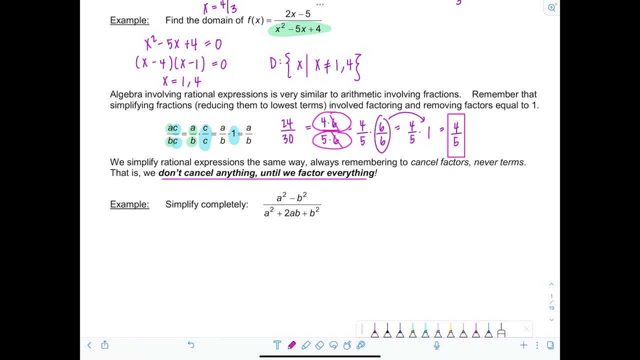 anything until we factor everything. so the numerator needs to just be a bunch of parentheses- see a factored expressions and denominator. also parentheses, doesn't matter how many there are, it's just no. canceling happens when you're in this land, right here. uh, it is not cancel time, because I'll tell you the most common thing I see: students. 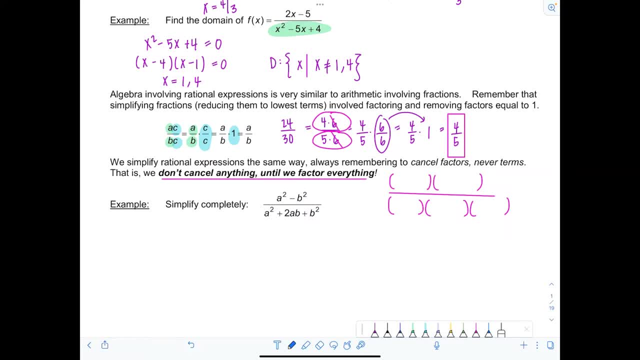 do they get so excited? because canceling is pretty fun, right? you're like B squared, bam bam. no, mm-hmm, don't even think about it, that's illegal math maneuver. the math police are gonna come after you real quick, okay, so here we go, the directions. tell us to simplify. 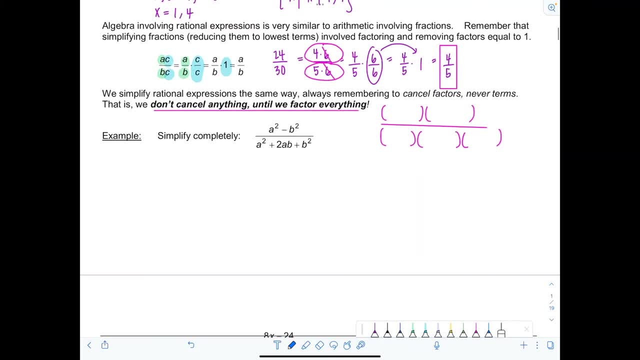 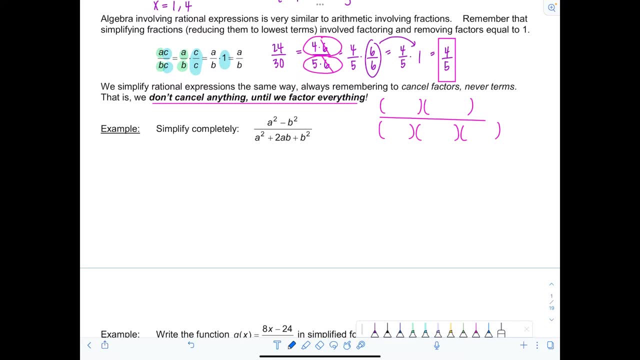 completely. we've got a squared minus B squared over a squared plus two AB plus B squared. so we've got to factor. if you're rusty on factoring, I'll link some videos here. I have a whole review playlist on factoring and I'll link it. 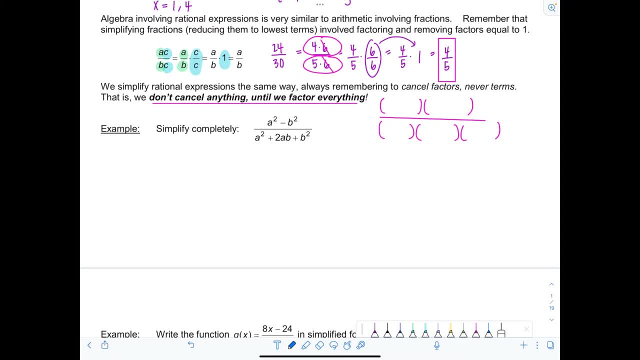 in the description too. so the numerator I recognize right away. it's a difference of squares: a squared minus B squared, so So that's going to factor into a plus b times a minus b. And then the denominator also. I noticed that's a perfect square trinomial. 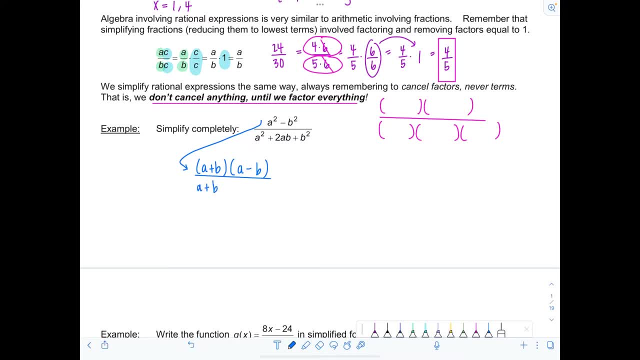 So that's a squared plus 2ab plus b squared. That's going to factor into a plus b squared. I'm going to write it out twice just to make it a little easier for the next step. And now you see how the rational expression is fully factored right. 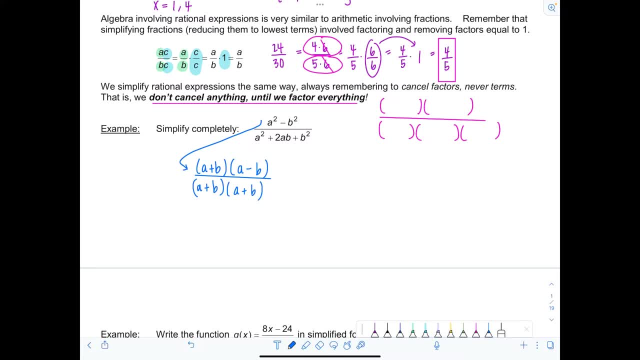 The numerator is factored, denominator is factored, So we can go ahead and start canceling any common factors that we see. Do you notice anything? we can cancel? Yep, I can cancel out a plus b from both the numerator and the denominator. 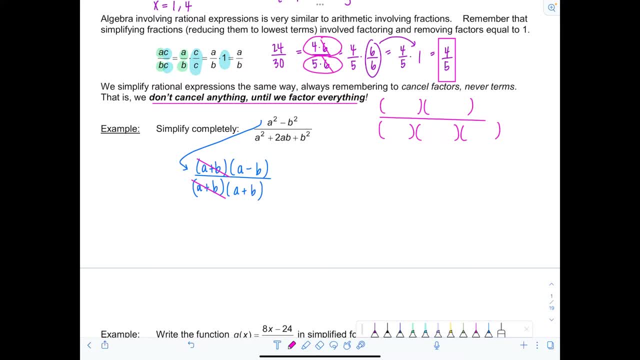 Anything else, No right. A minus b. that factor cannot be canceled out unless I had a minus b, A minus b on the other side of the fraction, on the other side of the in the denominator. Just because you have a plus b and it involves a's and b's, it's not the same thing. 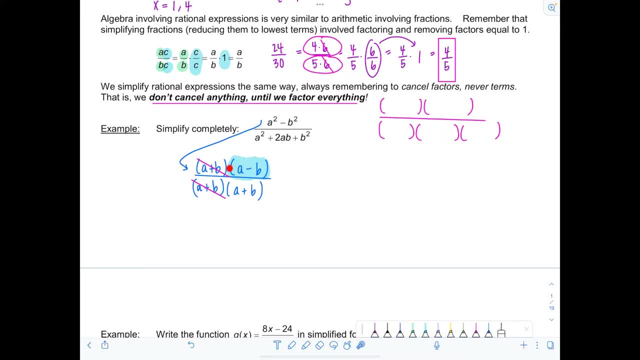 And you see how a minus b it's in there, grouped all happy in those parentheses, like a little family. So you can't go in there and start breaking them up, okay, Don't be a little homewrecker, So just leave it alone. 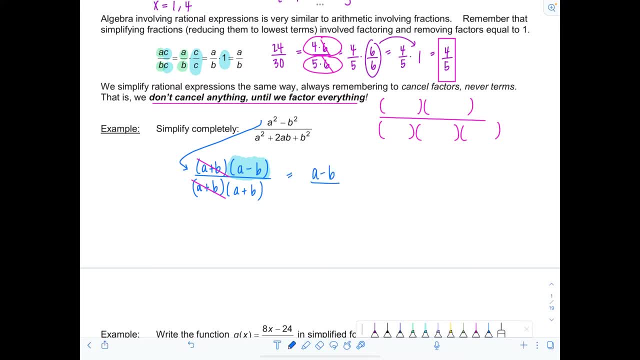 This is for our final answer: a minus b over a plus b, And you're done, okay. So, uh-uh, none of that, Don't even think about it. Just box it If you want to imagine that the parentheses are still there, right? 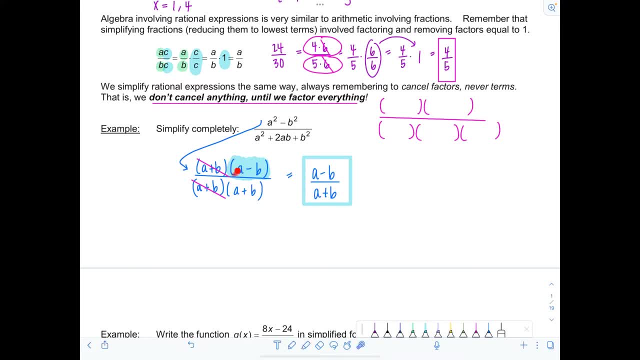 Just like they were. at this step. the parentheses are still there. We just don't write them when there's only one factor left over. They're still there, okay, So no extra canceling can happen. Good, good, good. Let's look at another example here. 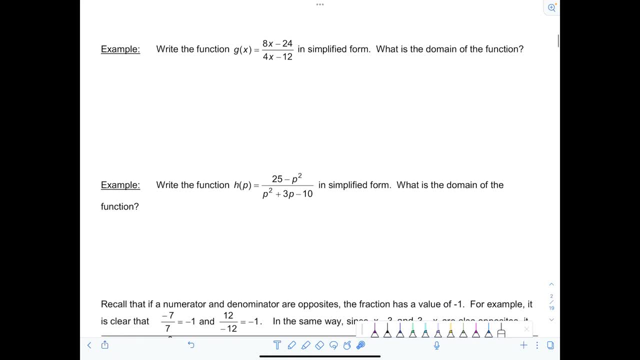 We've got a rational function, this time G of x, and we're asked to write it in simplified form and find the domain of the function. Okay, so to write g of x in simplified form. I want a factor, numerator, denominator and. 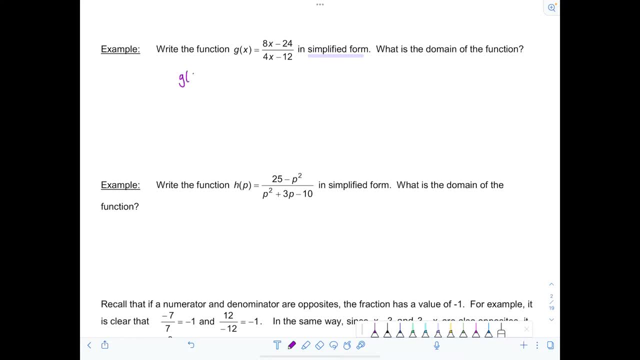 see if we can simplify any. So g of x. let's see Anything you notice about the numerator 8x minus 24.. We can take an 8 out right from both terms. So we have 8. 8 times x minus 3.. 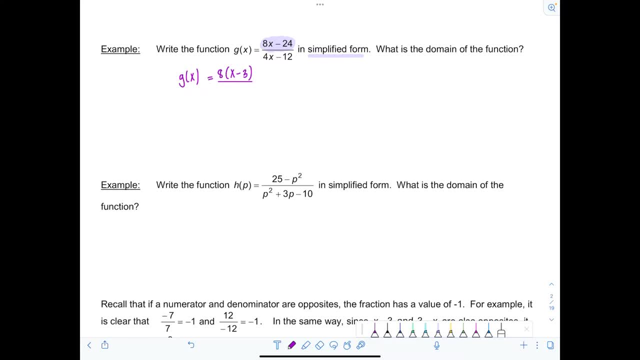 And then what about the denominator 4x minus 12.. Well, we can factor out a 4 from both those terms, so we've got 4 times x minus 3.. Ooh, nice, Okay, anything you notice we can cancel. 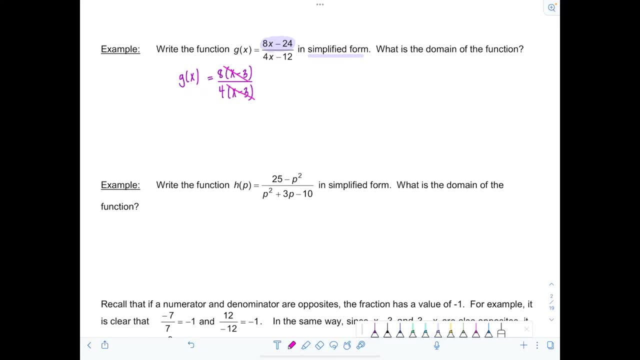 Yep, that x minus 3.. So bam bam, it's gone. And then now I'm just left with g of x is equal to 8x, 8 over 4. And 8 over 4 is actually not completely simplified. 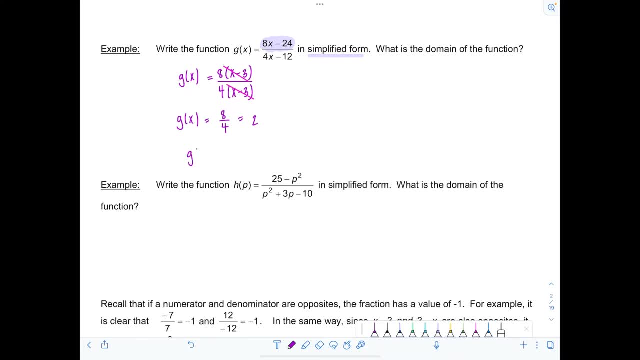 That reduces to 2.. So we can say g of x is equal to 2.. However, remember we were also asked to find the domain of the function, And any time that happens, especially with a rational function, you want to use the original. 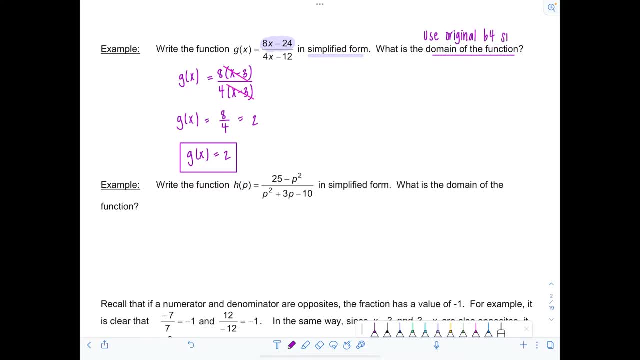 before you simplified. Okay, and you're going to see why right now. So if you look at the original way g of x was written before we simplified, it was a rational function with variables in the denominator, And I want you to pay attention right here that we actually did have a restriction that 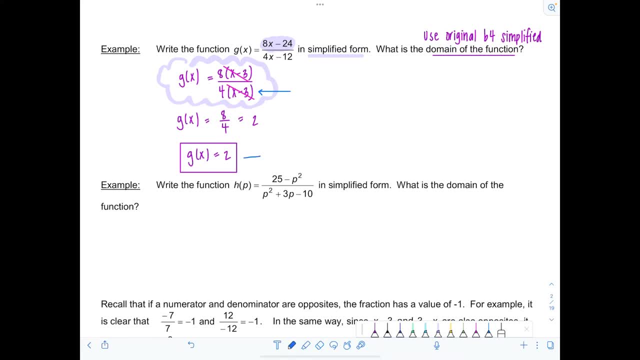 you don't notice anymore after simplifying. Okay, so looking at the original g of x. what restriction? Okay, so looking at the original g of x. what restriction? Okay, so looking at the original g of x. what restriction or what value did we need? 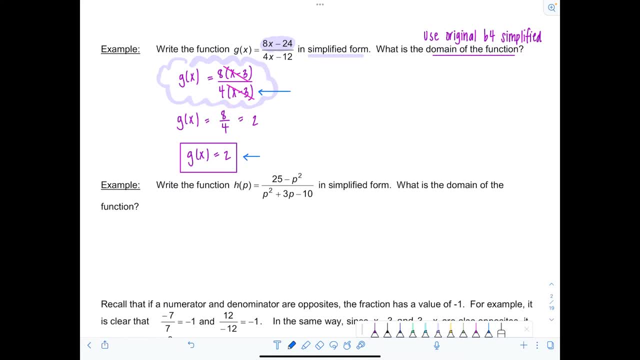 to remove from the domain. You see how we had 4 times x minus 3? Well, I don't want that to equal 0. So that means x cannot equal 3.. So the domain for g of x would be all x's, such that x cannot equal 3.. 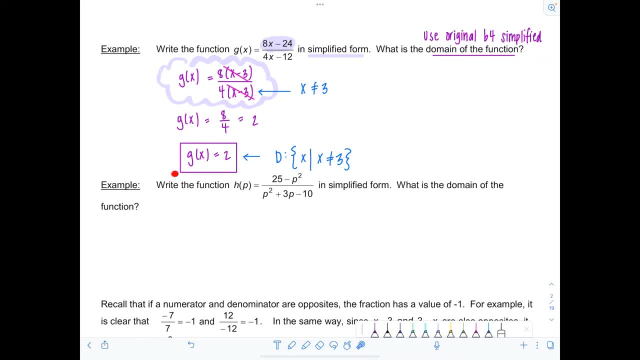 However, you wouldn't notice that if you looked at the simplified form of g of x, right Kind of dangerous. So make sure when you're asked to find the domain of a function and when you're dealing with a rational function, you want to use the original way the function was written. 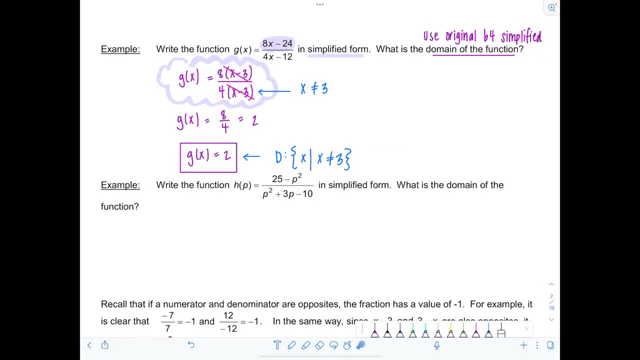 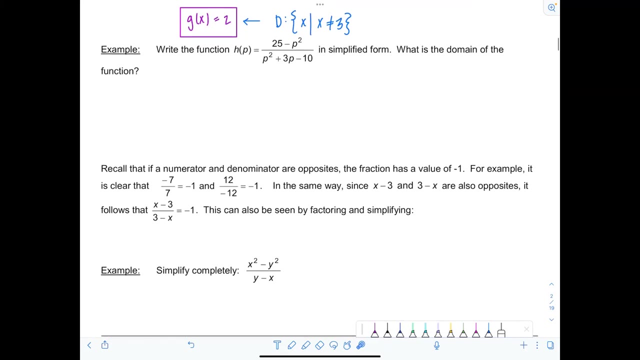 so you don't miss any restrictions that might be there. Okay, good, Let's look at another example. Write the function h of p in simplified form, and then: what is the domain of the function? All right, why don't you pause for a second? 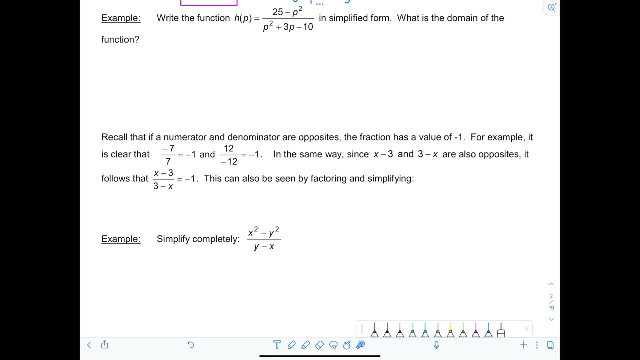 Pause the video. give this one a try on your own, and then we'll go over the answer in a minute. Okay, did you get it? Let's see. So h of p is equal to. before I simplify and start canceling, we've got to factor everything. 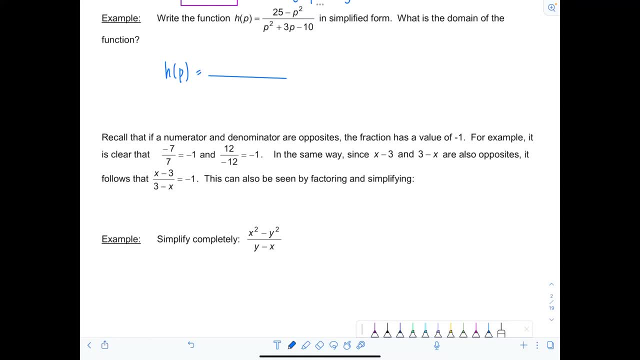 Now please be careful. You see how the numerator is 25 minus p squared. That's a difference of squares. It's going to factor into 5 minus p times, 5 plus p, Not p minus 5, p plus 5.. 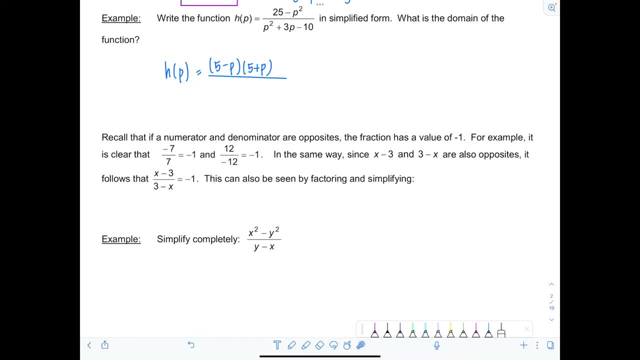 Okay, if 25 comes first, then that means the 5s have to come first in the factors and then the p comes second, since it was minus p squared. If you get the order wrong, it won't give you the correct result in the end. 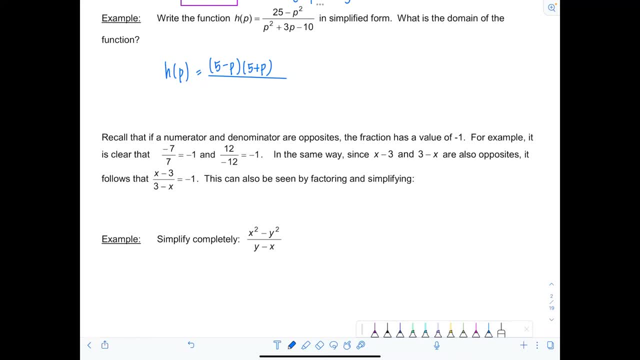 Oh no, And then denominator p squared plus 3, p minus 10, that's going to factor into p plus 5 times p minus 2.. Okay, anything you notice we can cancel. Why yes, p plus 5 is actually the same as 5 plus p. 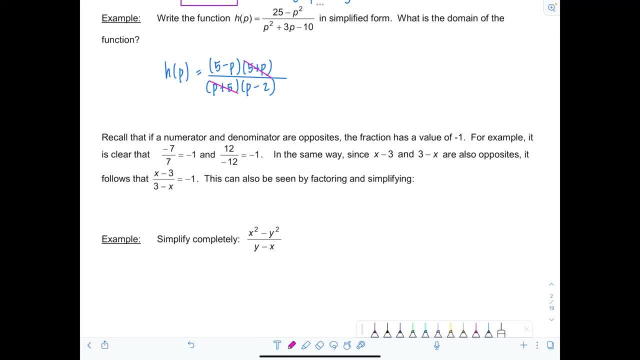 Remember, addition is commutative, So you can switch around the order when you're adding two things, not with subtraction, though You can't do that when you're subtracting two quantities. So if the order switched up when you're adding in those little parentheses, no big deal. 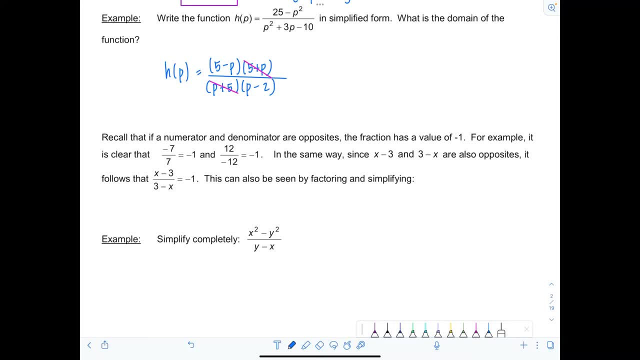 You can cancel, And so now we're left with h If p is equal to 5 minus p over p minus 2.. Can I cancel out those p's? It's just so tempting. I love canceling. It's my favorite thing ever. 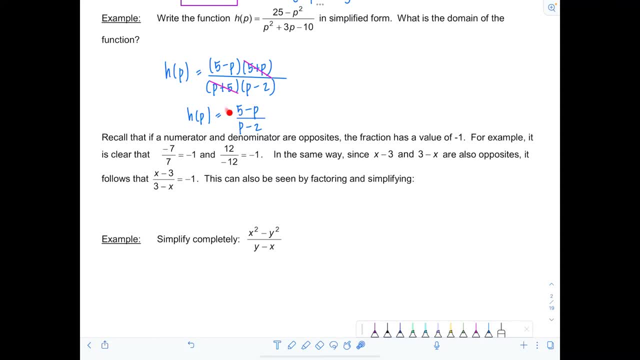 I hope you're yelling no over there. right, 5 minus p is a factor all on its own. It's a little family. See it hanging out so happy in the parentheses here. We don't need to put it in the last step, but that stays together. 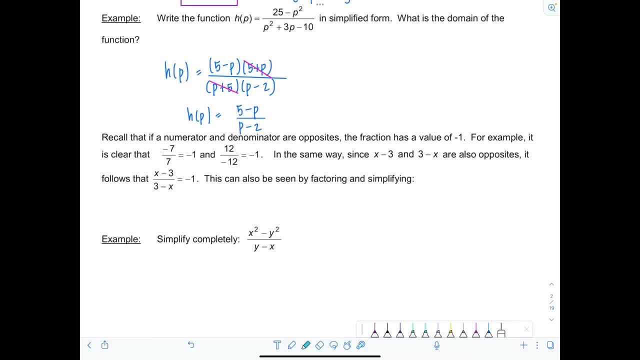 And p minus 2, that's another factor. No more Canceling. We did all the canceling we could, So there we go. OK, now we're asked to do something else. We're asked to find the domain of the function. 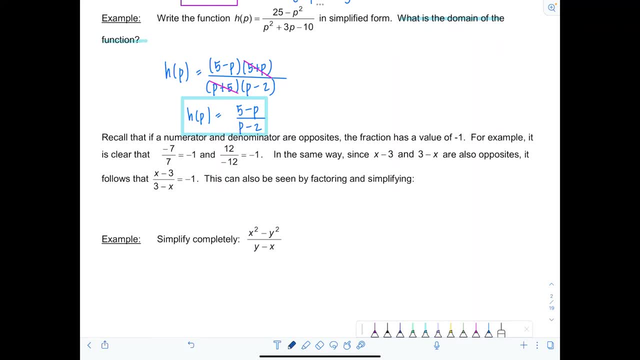 So remember, you're going to look at the original when you're finding the domain, so you don't miss any restrictions. So what would make the denominator zero? What would make h of p undefined if p plus 5 or if p minus 2 was equal? 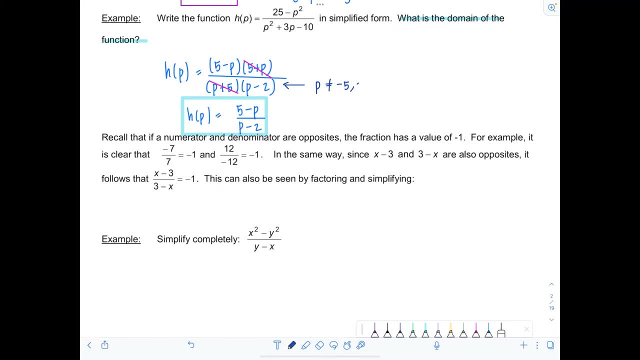 So that means p cannot equal negative 5 or 2.. So when I write the domain, we're not using x's with this function. How funky. OK, the domain is all p's, such that p cannot equal negative 5 or 2.. 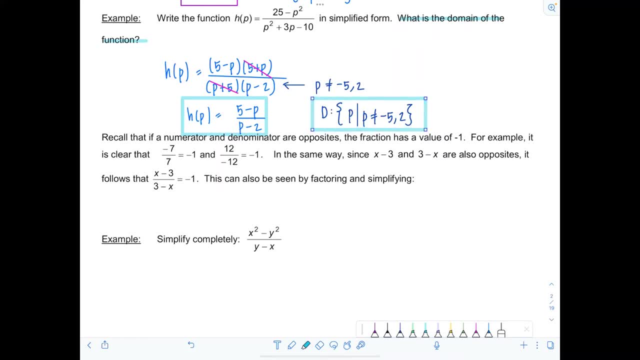 And that is it Good. OK, now we talked about how addition is Commutative. earlier right, We discussed the fact that 5 plus p is the same as p plus 5. And I mentioned that's not the case with subtraction. 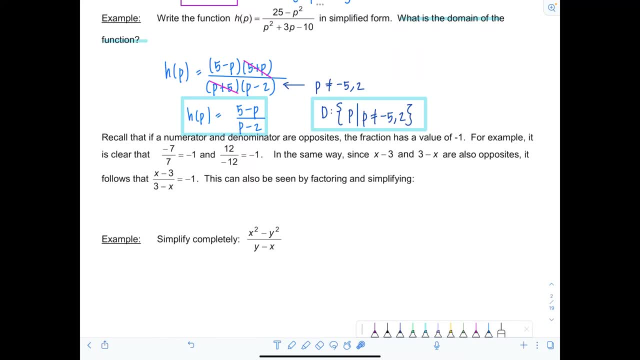 But there is kind of a cool way that we can simplify factors: if you have the same two terms and the order of subtraction is reversed. What am I talking about? You'll see right now. So when the numerator and denominator of a fraction are opposites, it has the value of negative 1.. 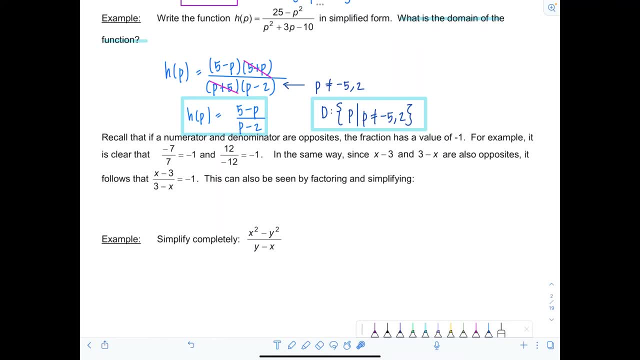 So think back when you were studying just how to work with fractions. If you had negative 7 divided by 7, that was equal to negative 1.. Or 12 divided by negative 12, that's negative 1.. So it doesn't matter if the numerator or the denominator is negative. 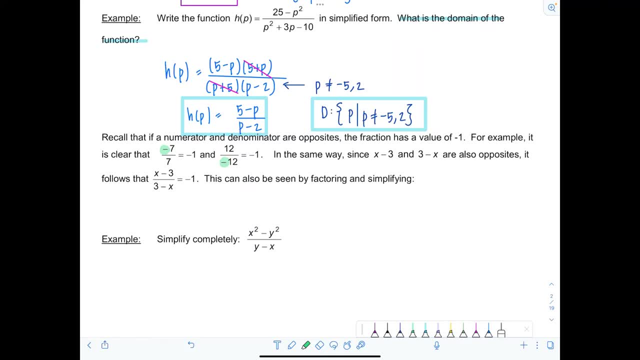 It's just as long as there's one negative either in the top or the bottom, not both, then your fraction is equal to negative 1. And 7 and negative 7 or 12. And negative 12 are opposites, in the same way that x minus 3 and 3 minus x are opposites. 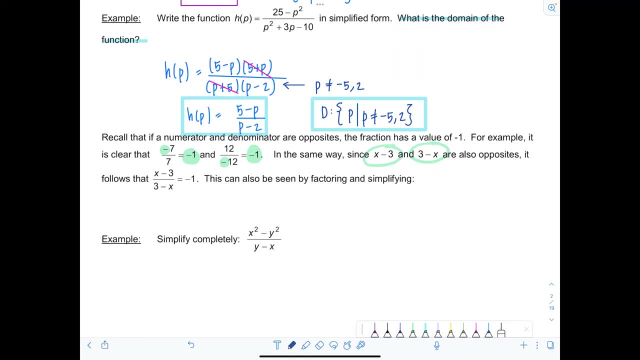 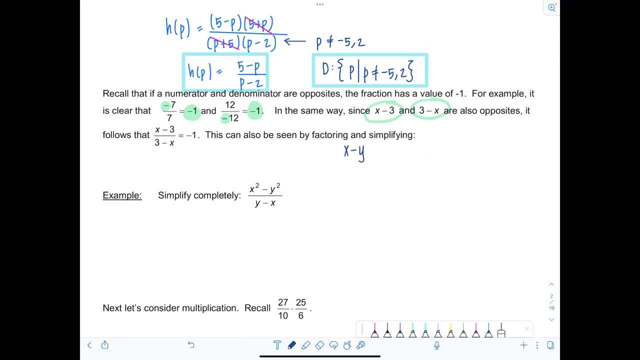 And for you to understand that this is the case, let me kind of walk you through something else. So, generally speaking, we can say that x minus y, divided by y minus x, is equal to negative 1.. If you don't believe me, let's see here: 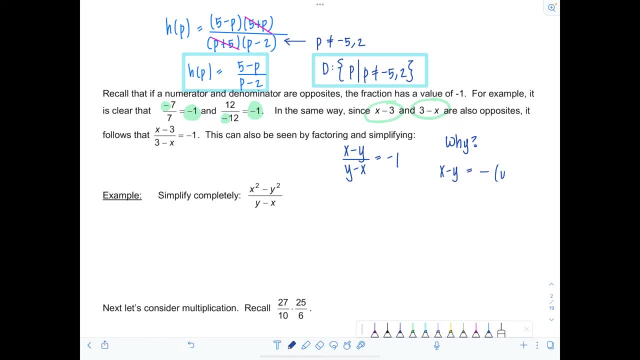 That's because x minus y is equal to negative y minus x. Let's check. Let's distribute this negative. We're going to check. Don't take whatever someone says as gospel. So we've got x minus y equals negative y plus x. 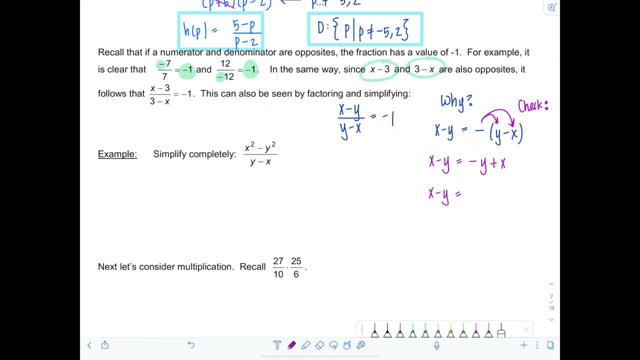 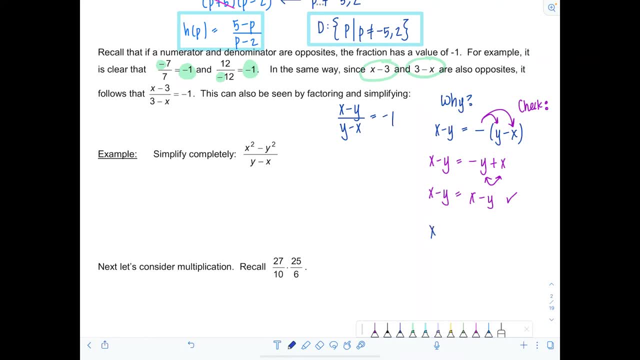 Okay, Okay, Okay, Okay, Okay. So we've established that x minus y is equal to negative y minus x. If I divide both sides by y minus x, notice here: this will cancel. This will cancel. I still have that negative left over. 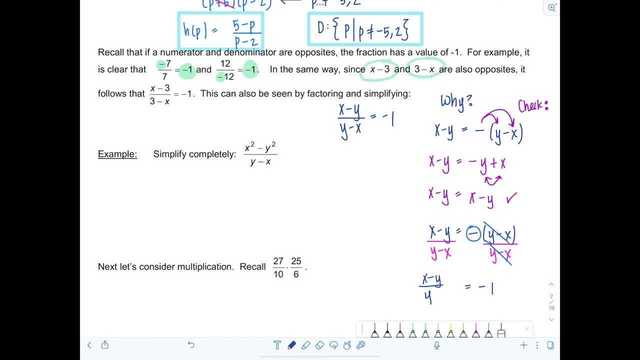 So I've got negative. 1 equals x minus y over y minus x. So this is going to be helpful for further canceling, in case you see that you have a factor in the numerator, factor in the denominator with the same two terms. It's just the order of subtractions reversed. You can go ahead and. 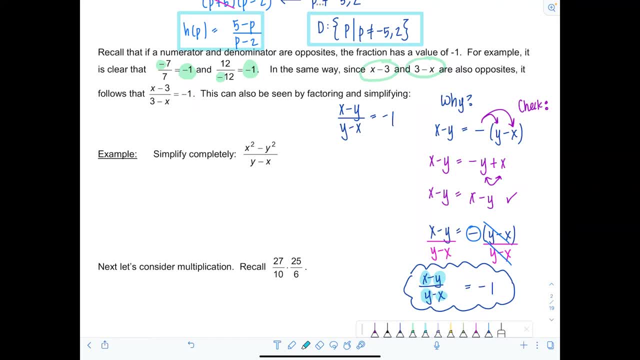 cancel. Just make sure you remember that's equal to negative one. So just add a minus sign, All right. So let's look here at this example. We've got x squared minus y, squared over y minus x. I can factor the numerator. It's going to factor into x plus y times x minus y. 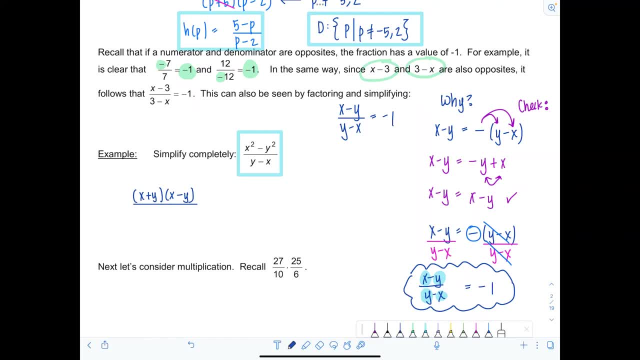 And then the denominator. that's all that there is to it. It's just y minus x. If you want to put parentheses around it, go for it. Okay, Now notice I can cancel out x minus y and y minus x, But remember that's equal to negative one. 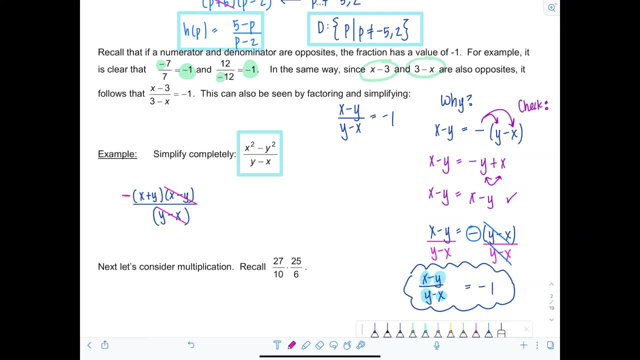 So I'm going to add a negative in my expression here and always put the minus one in the numerator, Don't put it in the denominator. So now we're going to be left with negative x plus y, which you could leave like that or distribute if you want: Negative x minus y. 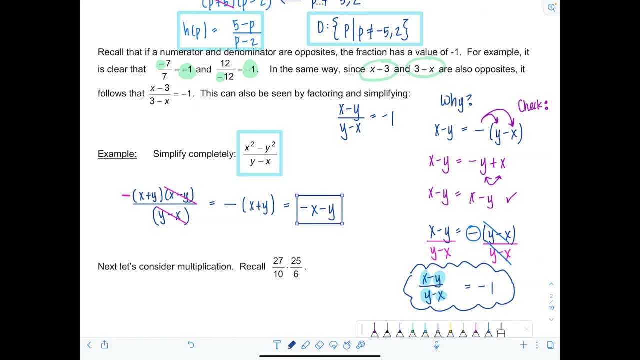 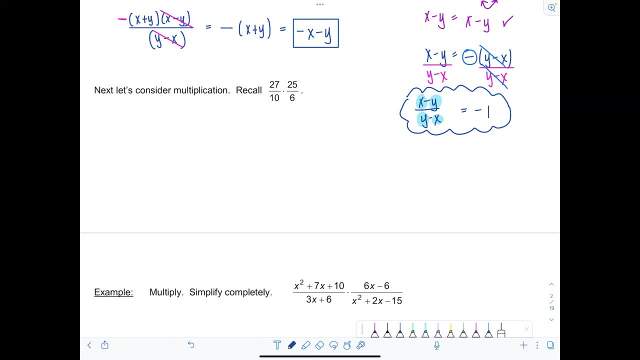 All right, Very good. Now we're going to look at multiplication. So how do we multiply rational expressions? Let's just look back to our rules of arithmetic when we were multiplying fractions. So say, you had something like 27 over 10 times 25 over 6.. 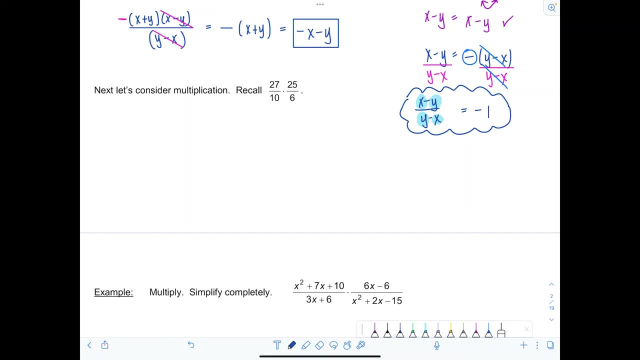 Bad idea is you sit there and multiply everything out: 27 times 25,, 10 times 6.. Instead, better way is to factor everything completely, So I'm going to go to the prime factorization. What am I talking about? 27 is 3 times 3 times 3, right? 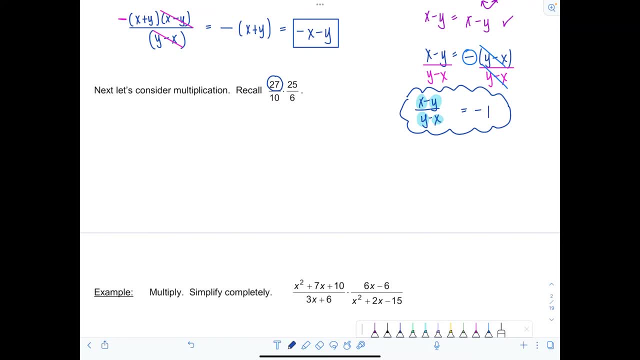 If you write it as a factor, using prime numbers, Okay, So 3 times 3 times 3.. And then 10 is 2 times 5.. 25 is 5 times 5. And 6 is 2 times 3.. 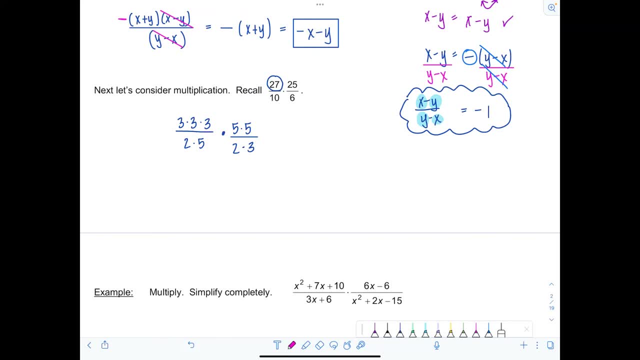 And then when you simplify, you cancel out any common factors So you don't have to stay within each fraction to cancel. If you see, say, a 3 in the numerator here and the denominator on the other fraction, that's totally cool. Cancel away Anything else. Oh yeah, These 5s right, Okay? 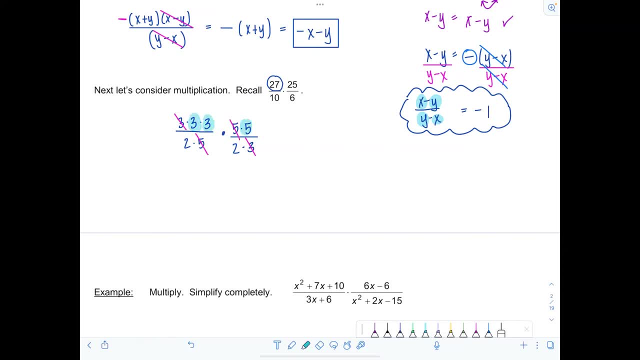 So what are we left with Now? we can multiply 3 times 3 times 5. That's 9 times 5.. So that's 45. And then in the denominator we've got 2 times 2. So that's 4.. And then we know, this is completely. 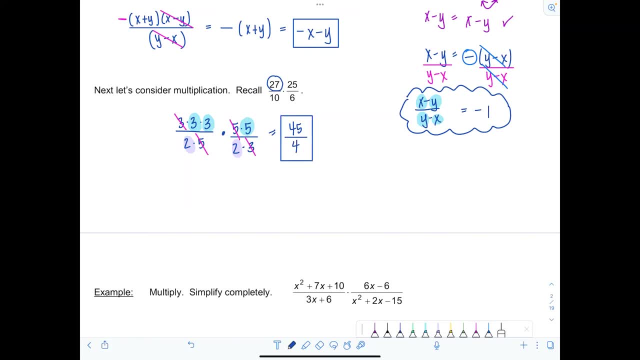 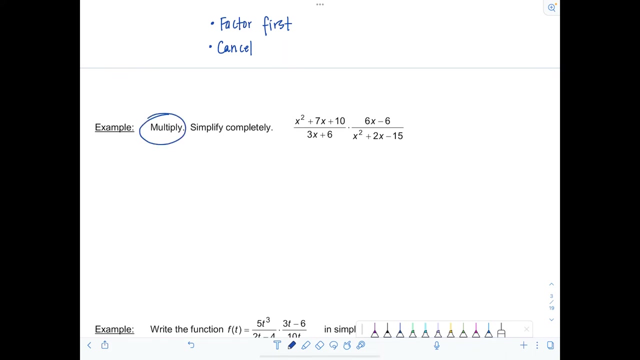 simplified. Okay, We canceled out all common factors. So just make sure you factor first, Then you can cancel And then you group everything together. So here we go: Multiply, completely simplify. Make sure you don't do this first. I know it's. 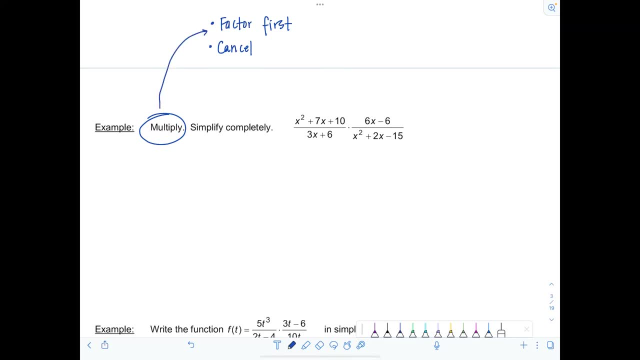 tempting. but you go: uh-uh, I know I'm supposed to factor first, then I cancel And then I'll do whatever multiplications left. So let's see, here We've got x squared minus 7x plus 10.. So that's going to factor into x plus 5 times x plus 2.. Now let's look down here: 3x plus. 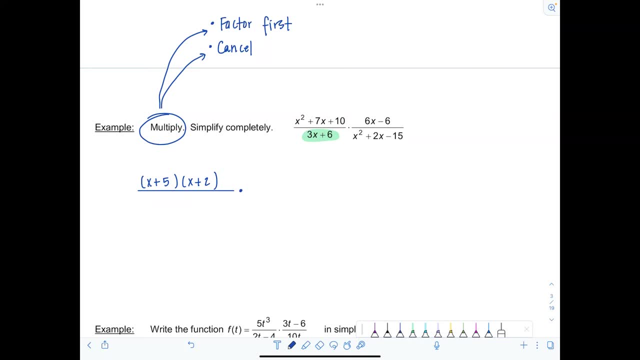 6.. I can take a 3 out, So I have 3 times x plus 2.. All right, Now let's look at 6x minus 6.. So I have minus 6.. What can you factor out of those two guys? Good, just a 6.. So I have 6 times x minus 1.. 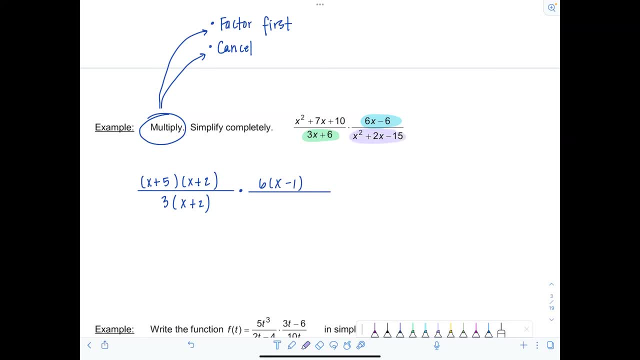 And then, last, we have x squared minus 2x plus 15.. So how's that factor Good, x plus 5 times x minus 3.. Lovely, So, now everything is factored, We can go ahead and start canceling out any common factors. It's time to have a cancel party, as I like to call it. So. 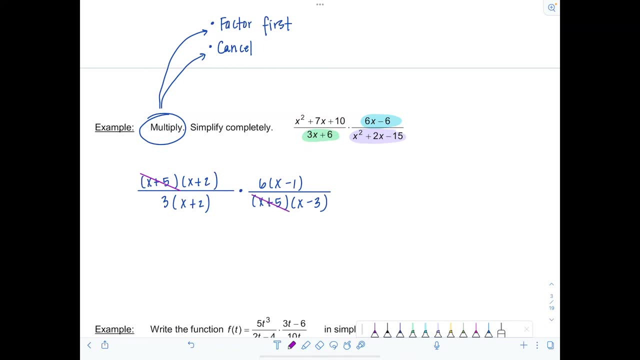 oh, look, here's x plus 5 in the numerator, x plus 5 in the denominator Cancel, cancel, What else? Yeah, x plus 2.. That's gone, Love it, Anything else? Yeah, how about the 6 and the 3?? So I can cancel out the 3 here. 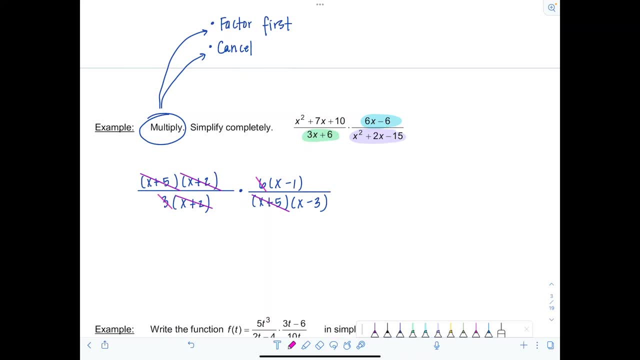 And then if I cancel out a 3 or divide by 3 from the 6, it's going to become a 2.. Very nice, So I think that's all we can do. Let's go ahead and write what's left over. So in the numerator we have 2 times x minus 1.. And then in the denominator 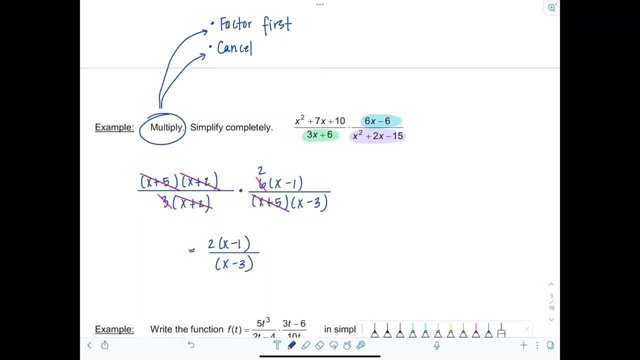 all I have now is x minus 3.. So I'm not going to leave the parentheses like that in the denominator. I just wanted to remind you that's a factor, And then, if you want, for your final answer, you can destroy it. And then, if you want, for your final answer, you can destroy it, And then 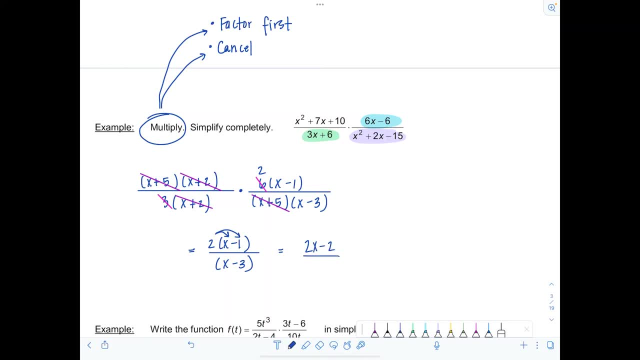 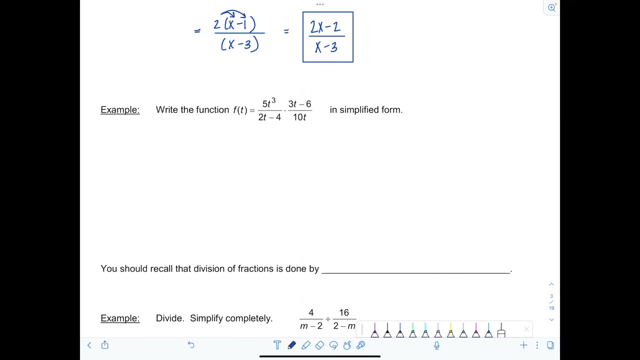 we'll distribute out the 2. So we'll have 2x minus 2 over x minus 3.. Very nice, How'd you do Good? Okay, let's look at another example here. So write: the function f of t equals 5t cubed over 2t minus 4 times 3t minus 6 over 10t in simplified. 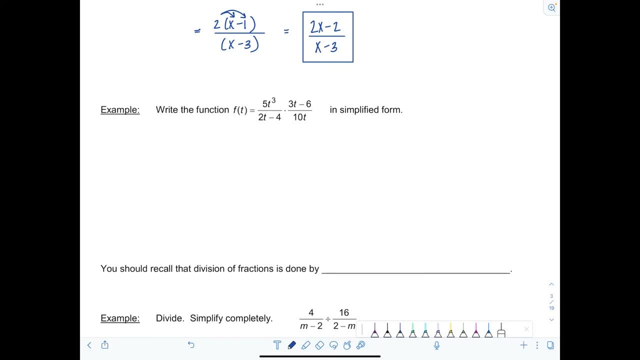 form. All right, very nice. So why don't you guys go ahead, pause the video? give this one a try, and then we'll go over the answer together in a minute. Okay, did you start by factoring? So f of t is 5t cubed over 2t minus 4.. You can take a 2 out. 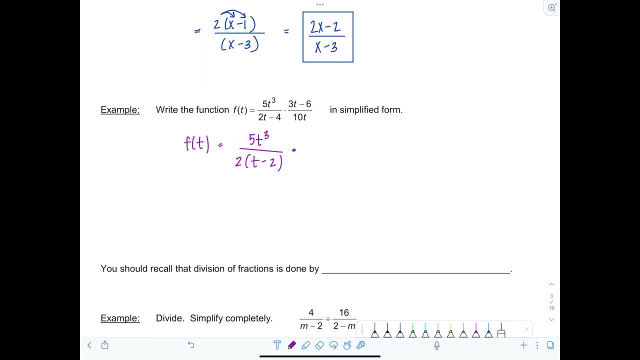 and then you have t minus 2 left, Good, Okay. and then 3t minus 6.. Again, I could take a 3 out, and then I have t minus 2, and then 10t is just hanging out in the denominator. 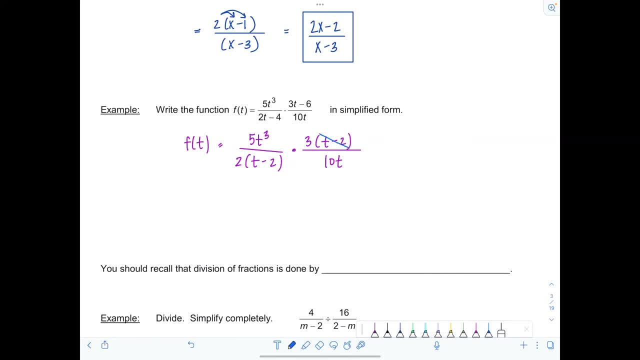 All right. so what can we cancel? First thing, I notice t minus 2, that's gone. Anything else? Yeah, the 5 I can cancel out, and now the 10 is going to become a 2.. And then also, did you catch this? 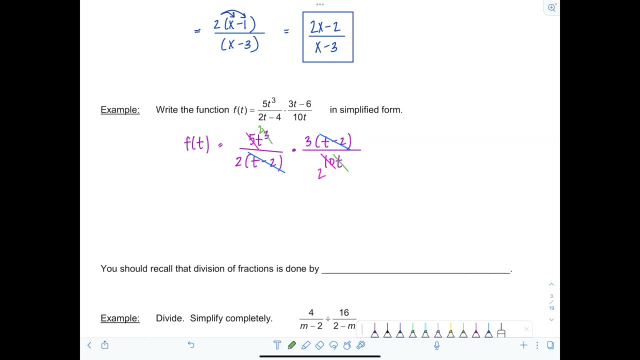 t cancels, and now I just have t squared in the numerator. Okay, so what's left over in the numerator? I've got 3 and a t squared, So 3t squared over what survived in the denominator, We've got a 2 and a 2.. So 2 times 2, that is 4.. Very good, So that is f of t in simplified. 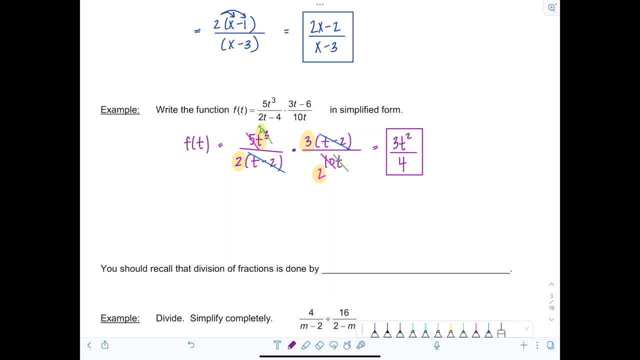 plus 1, right, So that was not equal to 4.. There was noef y, and that's a krypton. So the last number I'm going to provide is T plus 1x squared dollars. Okay, so you do big fractions, double on the dy and then you double D to get. 100.. We're going to round things out just here, just with a several key apertures: 0, I'm going to write dominæ 7x, which is 8xx. so if I were to write the domain, it would be all ts, which means it's. 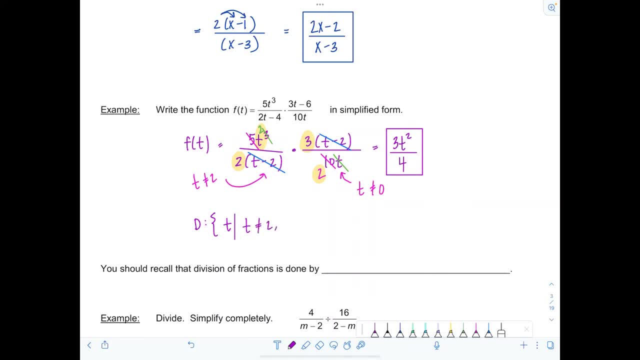 such that t cannot equal 2 or 0. You could put 0 and then 2,, 2 and then 0. It doesn't matter when you're listing restrictions, Okay, good. So now that we've got a handle on multiplication. 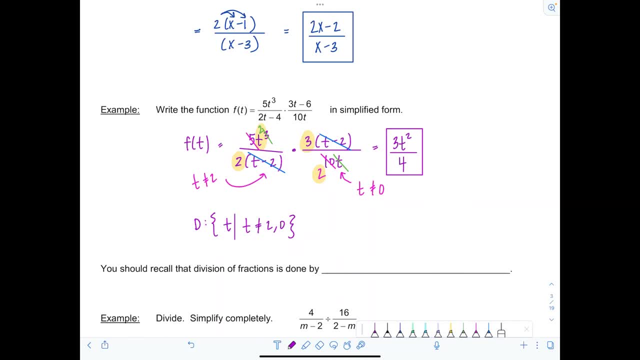 let's move on to division, And remember division of fractions is done by multiplication by the reciprocal. So remember, when you're dividing two fractions, if you have a over b, divided by c over d, you rewrote it as a over b times. 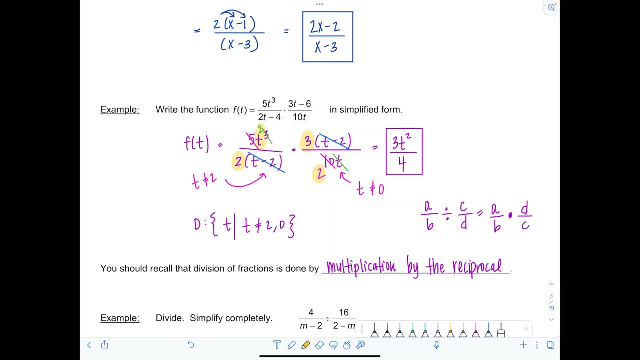 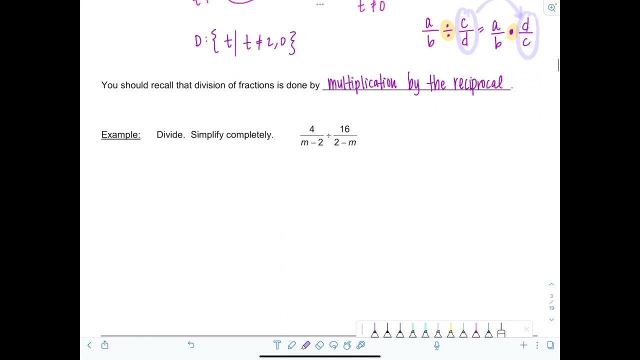 and you flip the second fraction. So you change division to multiplication and then the second fraction, the second rational expression, is going to get flipped, Okay. Okay, That's the reciprocal. So let's look at some division problems. It's not going to be that much different than multiplication. 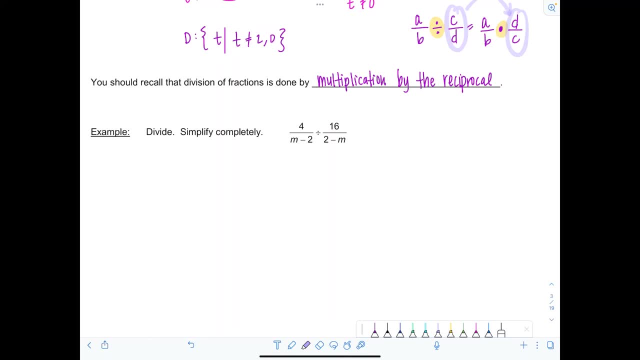 You just got to add that extra step in there. So divide, simplify completely. And again, when they tell you divide, you go uh-uh. I know I need to factor first. even though they don't remind me, I'm going to remember on my own. 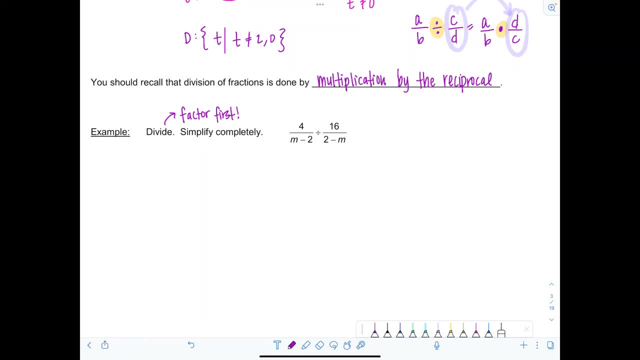 Here we go. So we have 4 over m minus 2, divided by 16 over 2, minus m. Okay, There's no factoring to do, Everything's factored, So we can just move on with our lives. So we have 4 over m minus 2.. 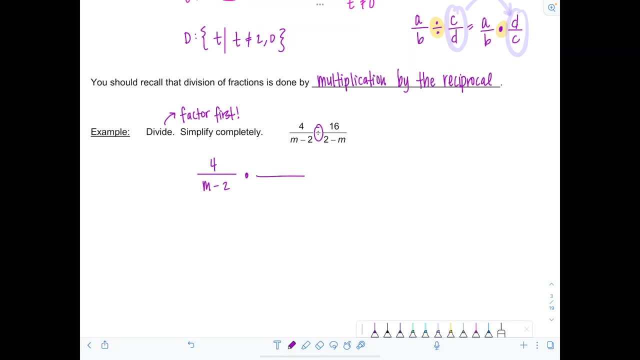 And then I'm going to rewrite this division as multiplication and flip the second expression, Not the first one, the second one. So we've got 2 minus m here and 16 down here. Good, good, Remember, this is a factor. 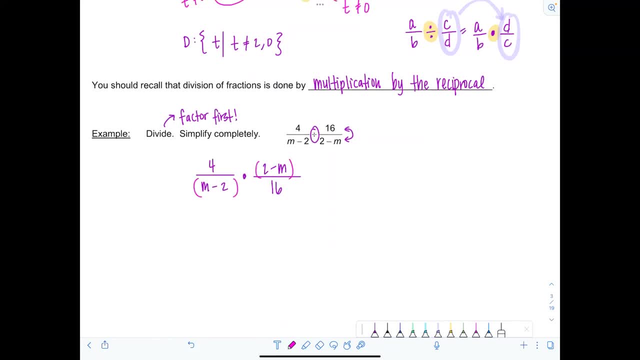 This is a factor, And 2 minus m, m minus 2, I can cancel those factors, But remember that is equal to negative 1 when the order of subtraction is reversed. So add a negative in the numerator And what are we left with now? 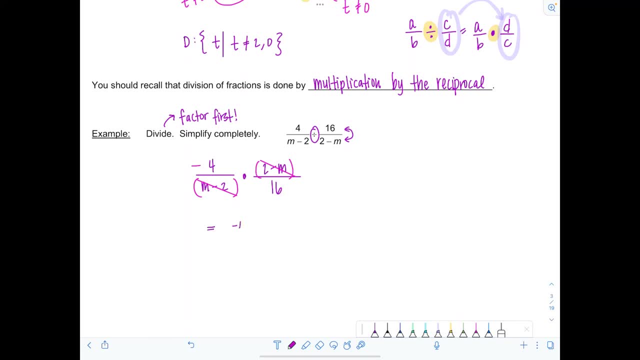 Oh, my goodness, We just have negative 4 over 16, which is negative 1. fourth, What's the original expression of this expression? Let me look at this. Wow, That means the original expression was just negative 1. person in disguise. 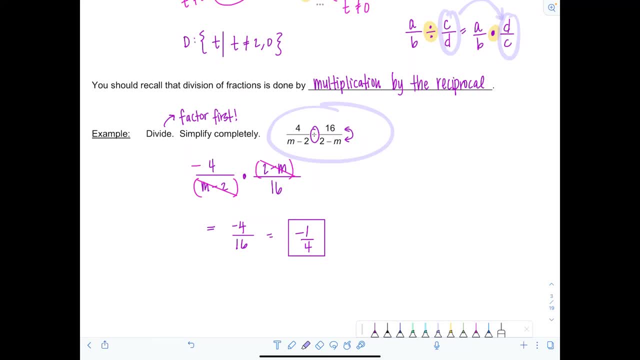 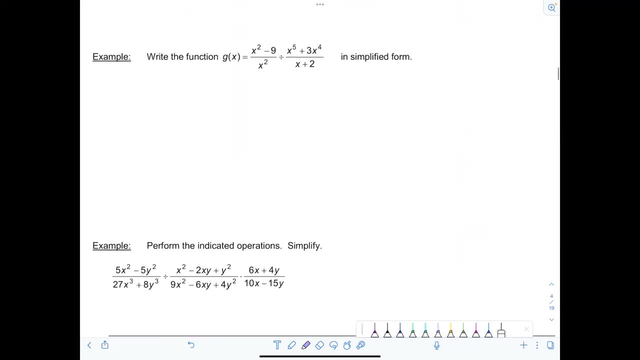 Who would have known? Okay, Let's look at something a little more tricky. huh, I think you guys are ready. Two more examples. So write the function g of x in simplified form, and then we're going to talk about the domain. 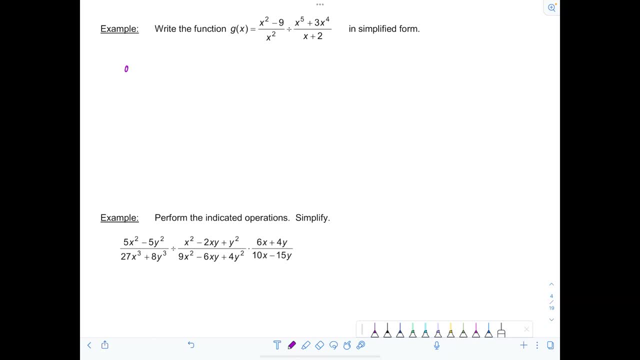 Okay, So here's: g of x. g of x is equal to x squared minus 9 over x squared. And then I'm going to rewrite the division as multiplication and then flip the second expression. So we've got x plus 2 over x to the 5th, plus 3x to the 4th. Okay, So now let's start factoring. 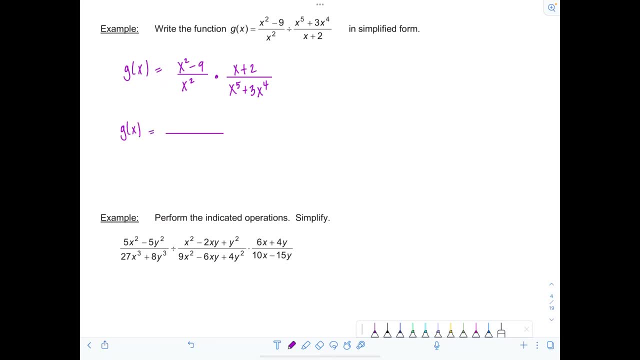 Okay, So g of x is going to equal. let's see x squared minus 9, that factors into x plus 3, x minus 3.. x squared in the denominator is just going to hang out there, x plus 2 in the numerator, nothing to do. I'll just put parentheses around it, so I remember I. 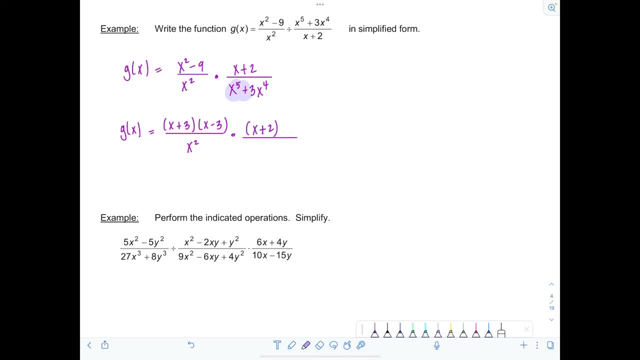 took care of it. Okay. And then look here: x to the 5th plus 3x to the 4th. What do they have in common? What can I take out from both those terms? Yep, I could take out x to the 4th, and then I have x plus 3 left. 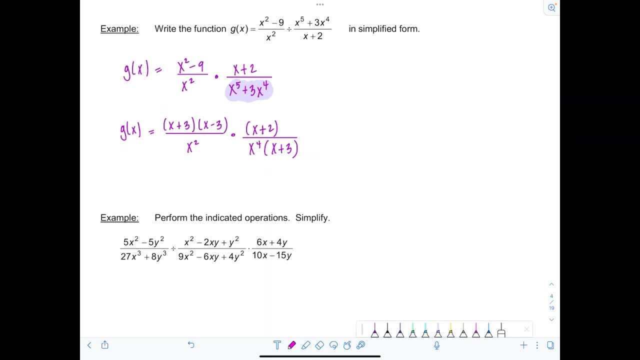 Okay, Good, Now it's cancel party time, So x plus 3 cancels Anything else. No, Oh, the party ended so soon. That was kind of a letdown. Okay, Now, what are we left with? So we've got g of x equals who survived the aftermath of the party. We've got x plus 3,. 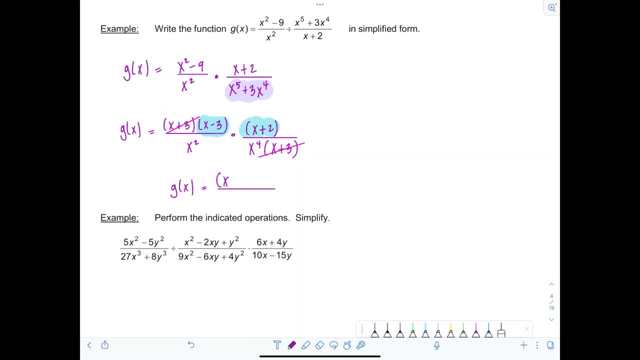 x plus 2.. Those are left over. I think I said x plus 3.. I meant x minus 3.. And then in the denominator, what do we have left? We've got x squared and x to the 4th, So that's going to give us x to the 6th. 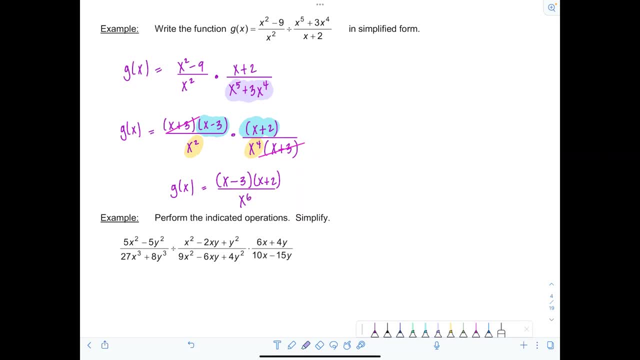 Now, if it was up to me, I'm fine if you just stop here. You don't have to foil out or multiply out everything in the numerator, but just check with your instructor. okay, if they care, I say stop here. 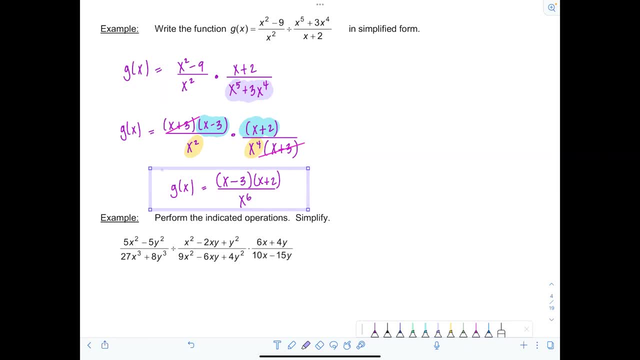 Stop while you're ahead, Okay, And then let's go ahead and find the domain. So when you're finding restrictions and you have to do some division, you have to be careful, because you've got a few places to look. You have to look in the original and also after you flipped. 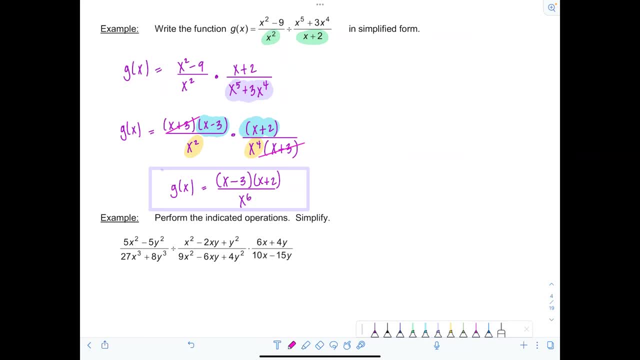 Mm-hmm, Mm-hmm. So originally, what restrictions do we see? Well, x squared, that means x can't be zero. X plus 2,, that means x can't equal negative 2.. And then remember, since we were dividing, we ended up flipping. 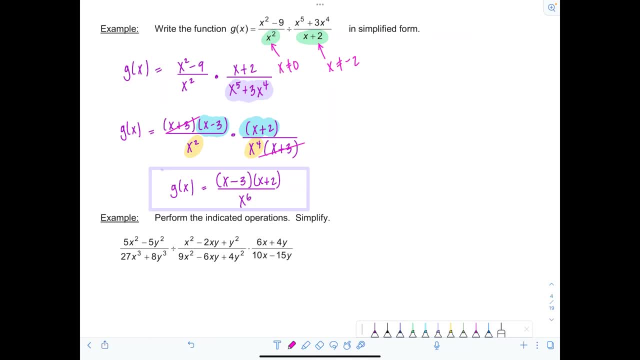 the second expression. Please look here. And then now we've got more restrictions. x to the 4th would be zero if x is zero. Well, I already listed that. But also x plus 3 would be zero if x is equal to negative 3.. So that's a third restriction. 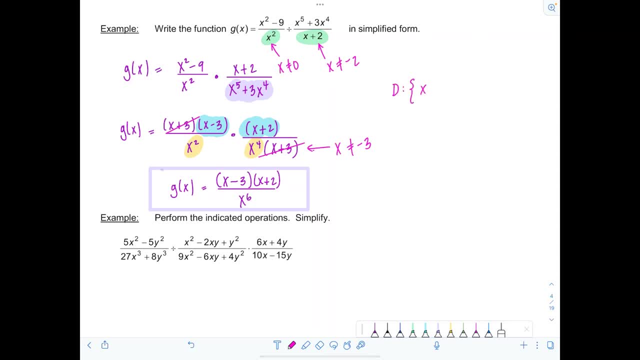 So that means my Domain is going to be all x's, such that x cannot equal zero, negative 2, or negative 3.. So here's kind of how it works When you have a rational function that involves division, right? So say you have f of x equals a over b, divided by c over d, and you're finding the domain. 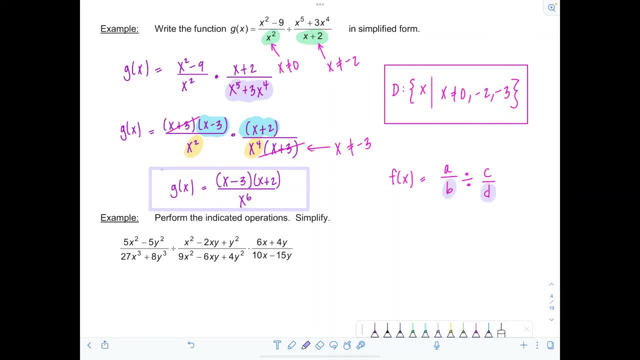 You've got to look for restrictions in the denominator of the original as well as the numerator of the second expression, because it ends up getting flipped or put in the denominator when you change it to multiplication. So those are the three places that you find restrictions. 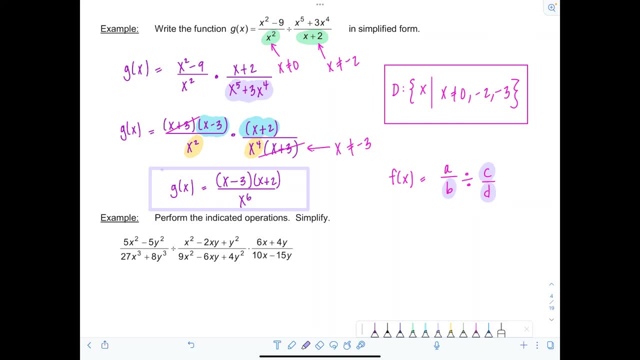 for your rational function, But it involves division, okay, Good, Now for the grand finale. look at this spicy little beast we've got Perform the indicated operation and simplify. Notice, we've got division going on with the first two and then multiplication. 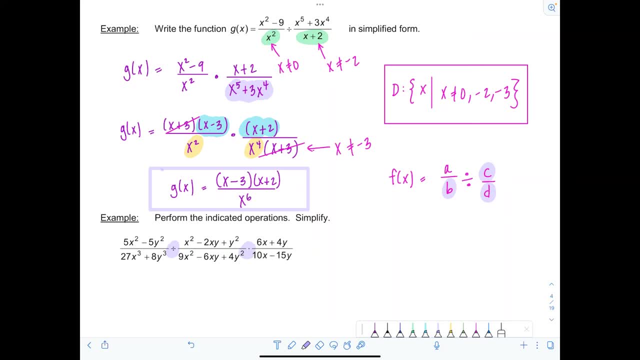 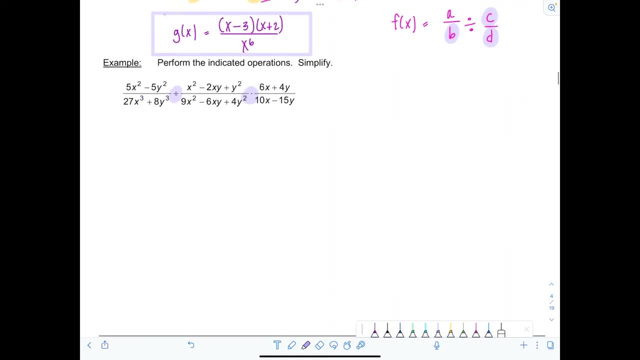 afterwards. So I hate PEMDAS because sometimes students think it means you have to multiply before you divide. but that's not true, okay. So when you're doing your order of operations, you do parentheses, exponents, then multiplication, division. They happen at the same level. You just 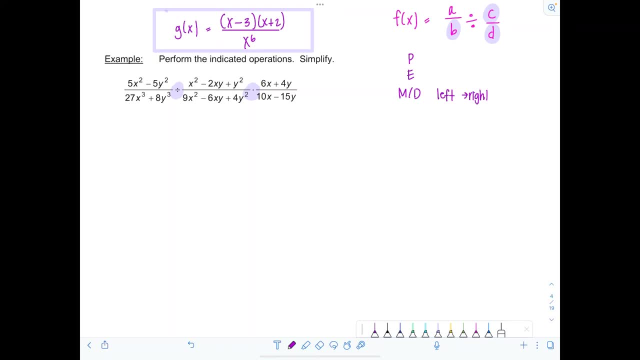 always work from left to right, Okay, and then addition, subtraction, same thing. So you would do any multiplying and dividing before you add and subtract. but as far as, do you do multiplication first, Do you do division first? You go left to right. okay, I'm just going to rewrite everything. 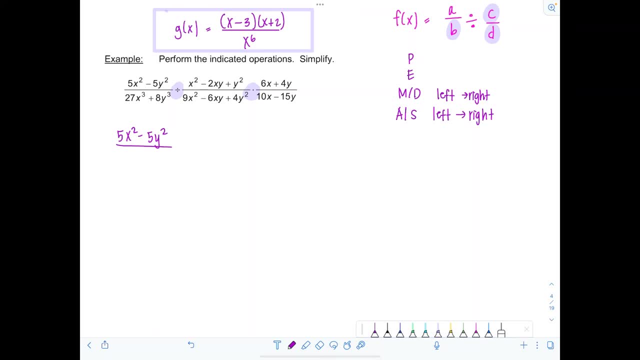 first and change the division to multiplication. okay, So you don't have to worry about it. So I'm not factoring just yet, If you want to go for it. So this is going to be times. and then 9x squared minus 6xy plus 4y, squared like that, over x squared minus 2xy plus y squared. 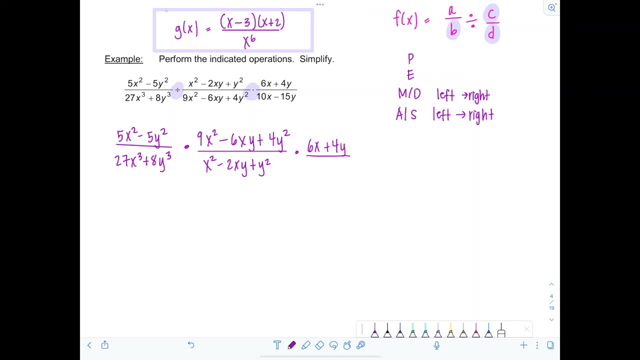 and then this one stays as is, okay, Then you don't have to sweat it. Good, good, good. Now let's go ahead and factor our little hearts out, okay, Just as a heads up for the first expression In the numerator, take the 5 out right, And then you have x squared minus y squared. 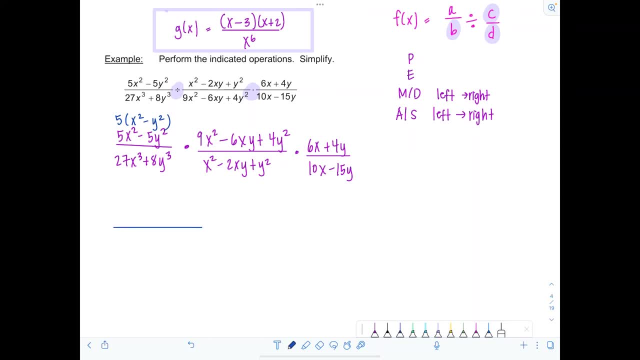 So that should help you get going there. x squared minus y squared, that's a difference of squares. so that's going to factor into x plus y times, x minus y, and you still have that 5 hanging out minding its business. 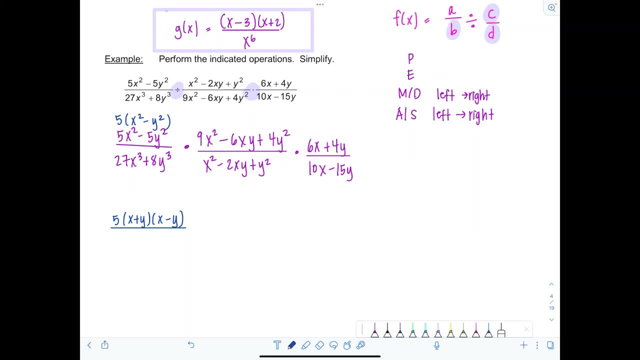 waiting for the cancel party. 5 showed up way too early. Okay, now we have 27x cubed plus 8y cubed. That's a sum of cubes. Do you remember how to factor a sum of cubes? No, Okay, I'll link a video here. 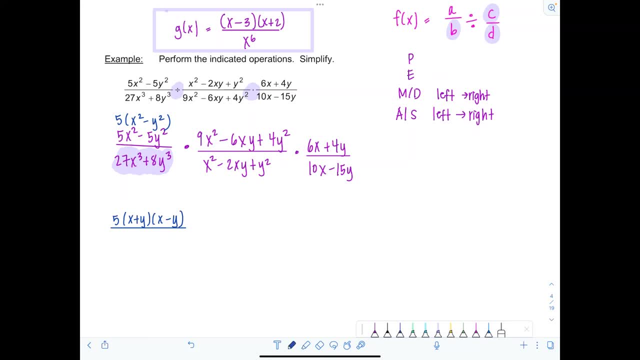 It's not too too like crazy. You just got to remember the pattern. So when you have a sum of cubes, it factors into a plus b times a squared minus ab plus b squared. okay, And you can use SOAP to remember the signs. 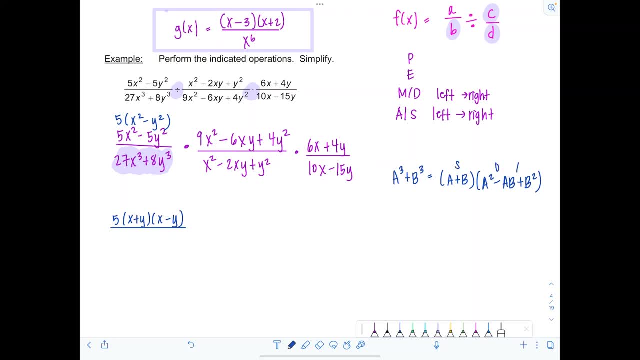 This is the same sign as the original. This is the opposite, and the last one's always positive. So in this case, a is equal to 3x and b is equal to 2y. right Since 27x cubed is a cubed. 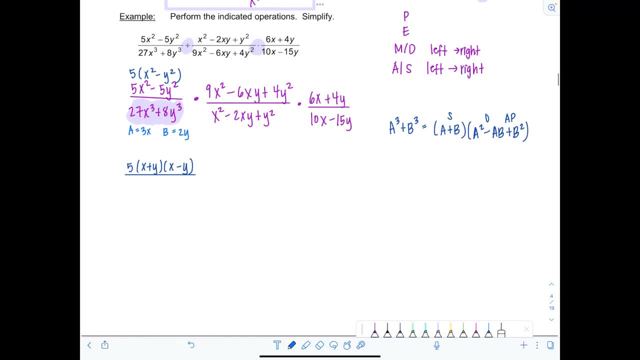 Okay, so to factor that, then let's see what we've got going on. We've got 3x plus 2y. 3x squared is going to be 9x squared Minus ab is 6xy. plus b squared is plus 4y squared. 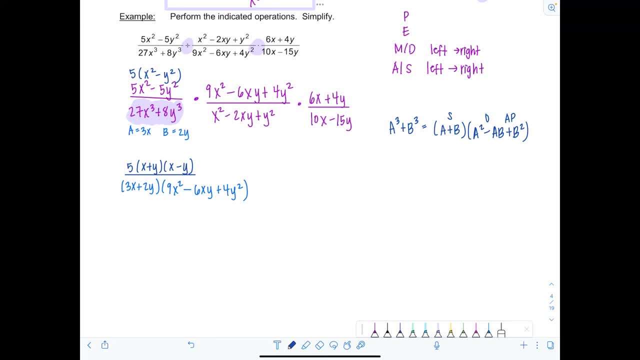 And if that's super confusing, then just watch the video on factoring a sum or difference of cubes, because I do break it down a lot more slowly if it's something you've never seen before. Okay times, Now let's move on to factoring the next expression. 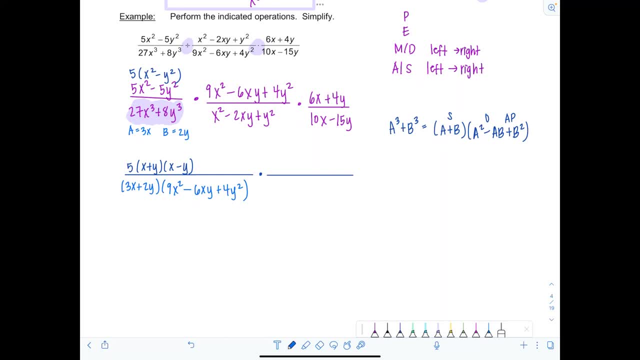 Just so you remember, when you factor a sum or difference of cubes, 99% of the time this thing is prime okay, So that means it can't be factored any further. So if I'm going to cancel this, it's because I'm going to see another factor. that's just like that. 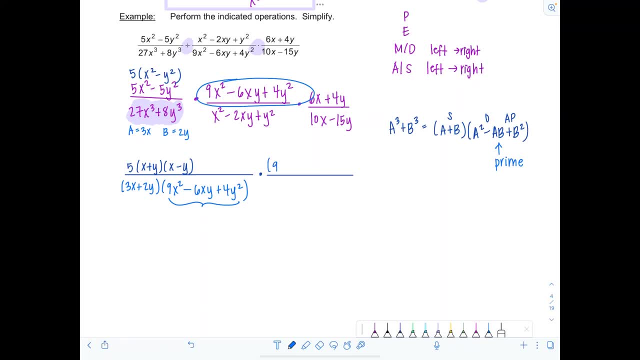 And lo and behold, oh my god, look, So that must be prime. I'm not going to waste any time trying to factor it. I'll get nowhere. And then in the denominator, let's see, we've got x squared minus 2xy, plus y squared. 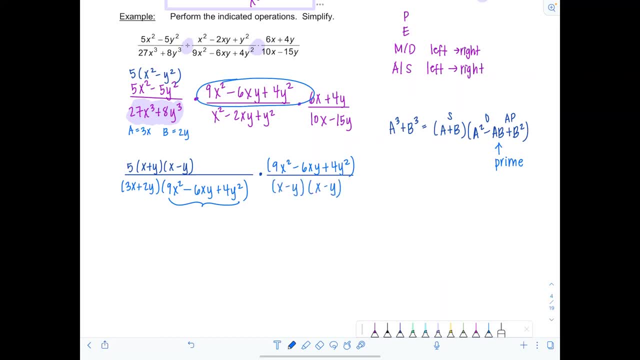 So that's just going to be x minus y times x minus y times 6x plus 4y. What can we take out from those two guys? Just a 2, right, So 2 times 3x plus 2y. 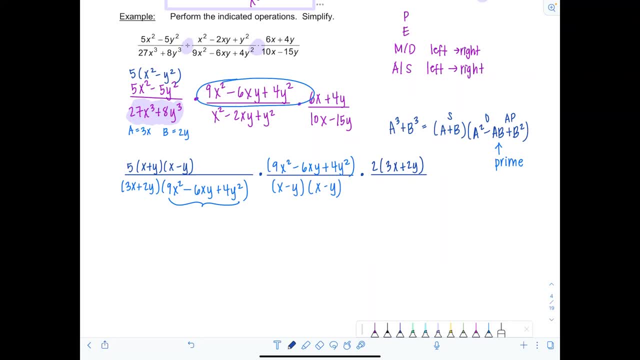 And then 10x minus 15y, we can take out a 5. And we've got 2x minus 3y. Okay, cool, Now it's cancel party time. Here we go. This one's satisfying right here. 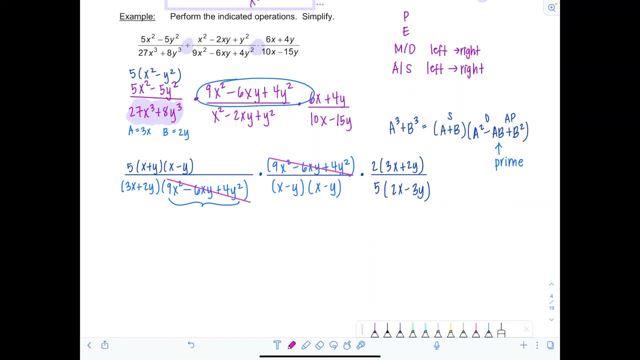 Bam, bam, be gone. What else? We've got x minus y over here and an x minus y over here. We've got a 3x plus 2y here, a 3x plus 2y here, Anything else. 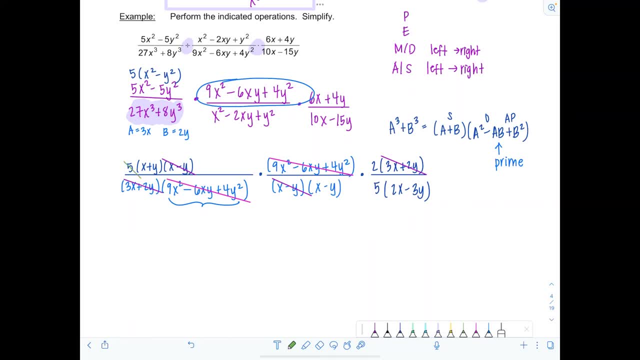 Yes, Look at this 5 is gone. This 5 is gone. My goodness, It was a massacre. Okay, so let's see who survived: x plus y and 2.. Aww, And then in the denominator we've got x minus y and 2x minus 3y. 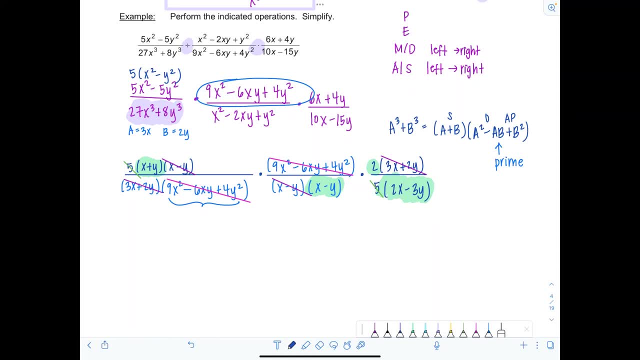 Aww, All right. so here we go In the numerator. we've got 2 times x plus y over. make this a little longer: x minus y times 2x minus 3y. You can leave it like that.